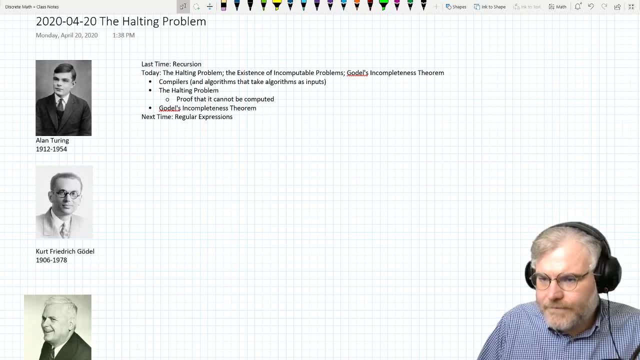 Let me fix that. So, as I said, chat as usual in Discord And there is the link to the chat in. I'm sorry, there's the link to the feed in Discord. Okay, So there's been some issues. Some people are saying they can't hear me. According to the system, people can't hear me. 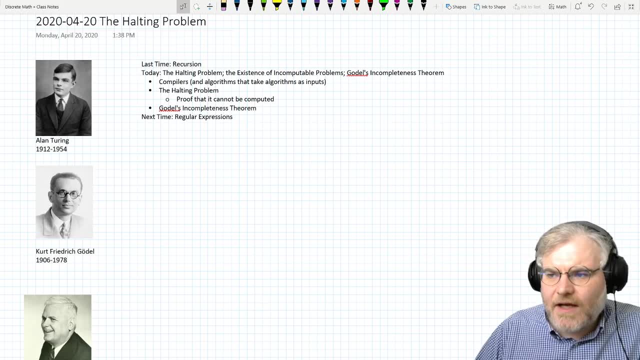 So there's been some issues. Some people are saying they can't hear me. According to the system, people can't hear me. If you can't hear me, please refresh your browser. Please check your volume. Is there anyone else that cannot hear me? 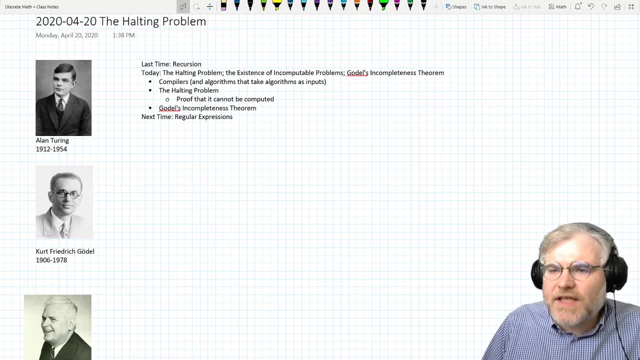 So okay. So today we're going to be talking about the halting problem. This is the last really big topic for the entire class. This is what we've been building up to when we're building up to recursion- Recursion, of course, being useful in and of itself, But today what we want to do is use recursion to show that there are things that, if my system can do- recursion. 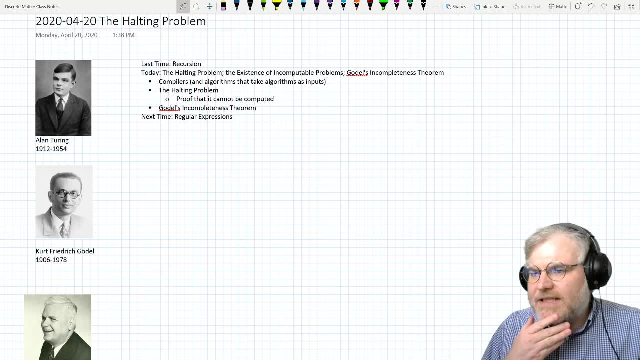 which Turing machines can, which computers can. that means that there are problems that I cannot compute Beyond, just the fact that there are things that I cannot enumerate and count. Okay, There are also countable things, and even you know things that should be. 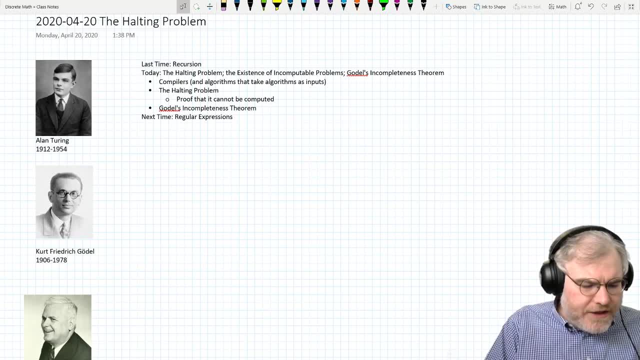 computable that you cannot. This is section. there's a good question. This is section. let me pull it up in the book. I had a bookmark in there. I hope I still have my bookmark, because my bookmark is where my notes are. 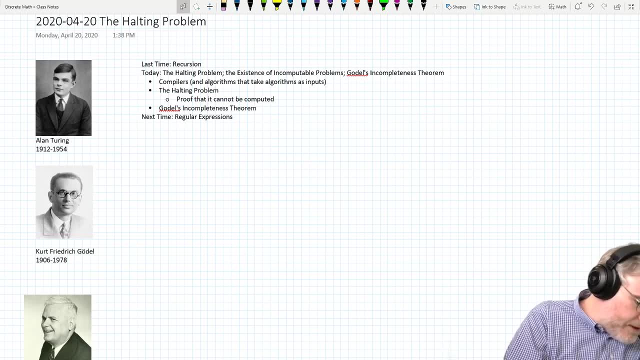 Oh, this is good. I lost my notes as well. Um, Here they are. This is section 6.4.. Boolean Algebras, Russell's Paradox and the Halting Problem. Okay, Of course we're not going to cover Boolean Algebras. That's cool, but it's beyond the scope of this course. 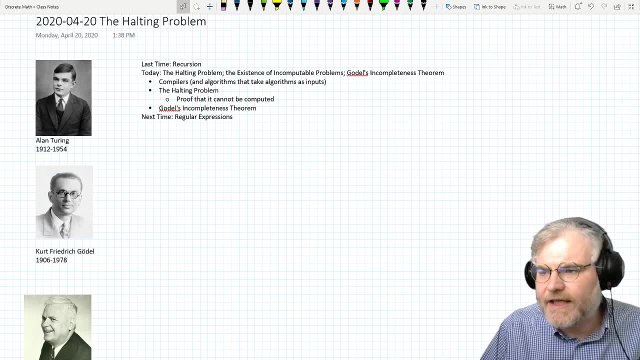 If you were a computer science major, you're, of course, covering it. What we want is: we want an intuitive understanding of the basic halting problem for this, and what we want is to talk about why recursion is important for this, And then we want to talk about Gödel's Incompleteness Theorem. 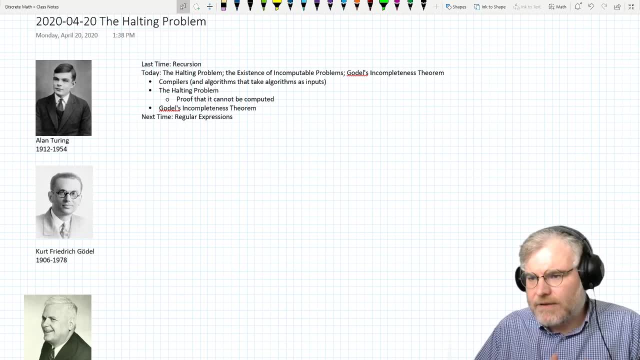 Okay, Next time I wanted to cover more about regular expressions. Next time I'm going to cover at least the beginning of what a regular expression is, because they're extremely important in IT And there are things that you can't do with regular expressions. 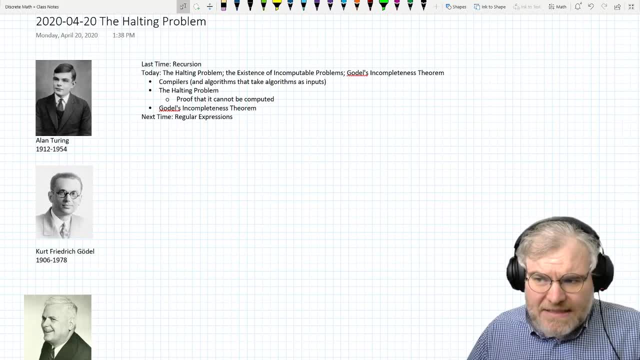 I want to talk about that. That may take two classes And if it does, that's the end of the course. If it doesn't take two classes, I will introduce I will- after introducing regular expressions. I will talk a little bit about P versus NP and why that's important to us. 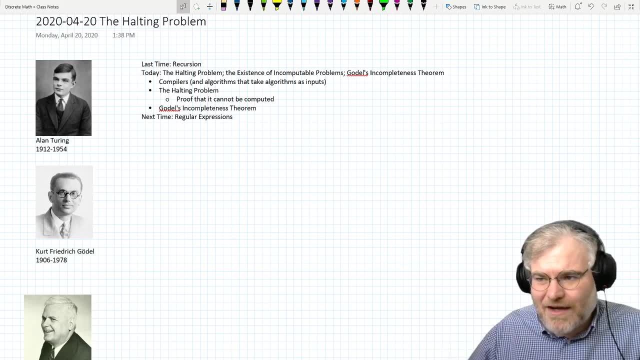 If we don't make it. I'm sorry, Stuff, I'm sorry to see go, but it has to go. Okay, Are there any questions other than that? Okay, So let's look at the quiz. You all just took a quiz. 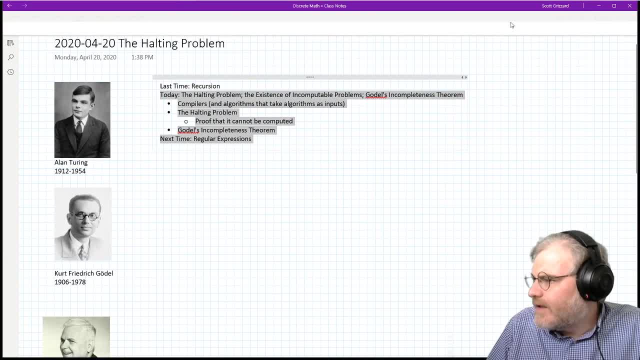 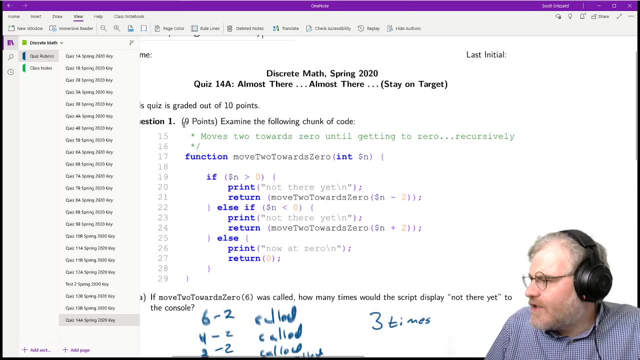 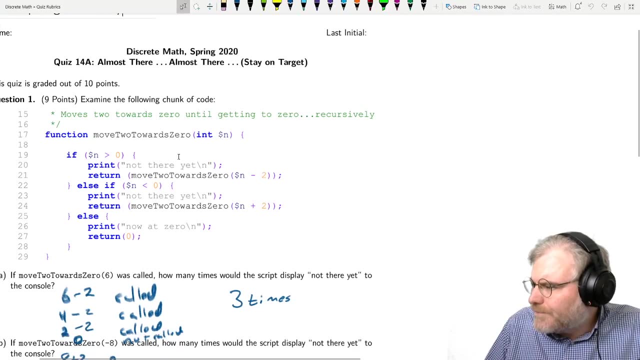 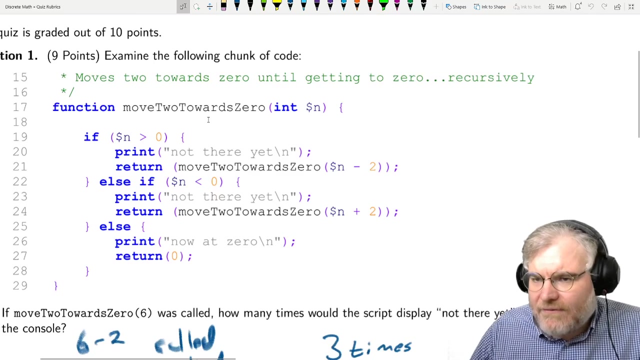 And it would help if I had the menu option to go to the quizzes. Okay, So you had a chunk of code And this code is a recursive function. Okay, So what happens here? I come in and I have a large string of ifs. 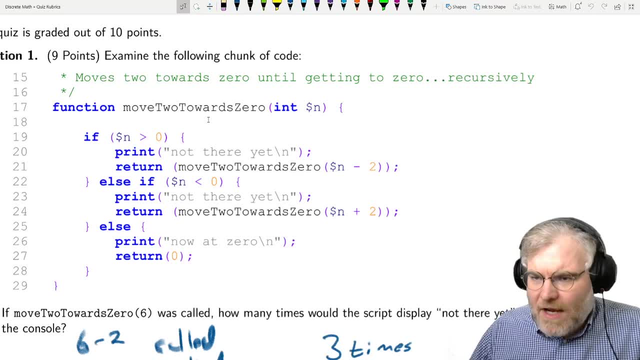 Okay, If n is greater than 0, I'm going to move 2 towards 0. So I'm going to subtract 2.. If n is less than 0, I'm going to move 2 towards 0, which means I'm going to go to pos in the other direction. 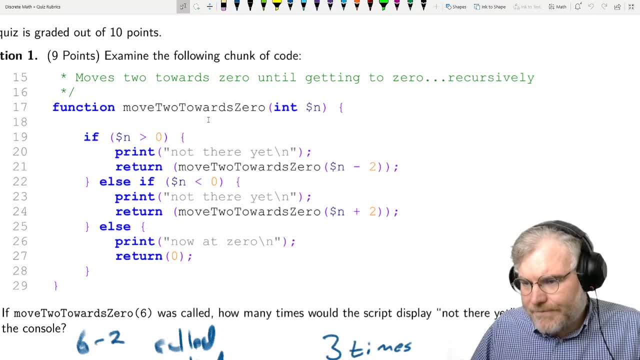 And if I'm at 0, then I'm done And I return: Okay, So 1 to 5.. Okay, So, what do we feel about this piece of code, what it's going to do? Okay, I guess I'll take another poll. 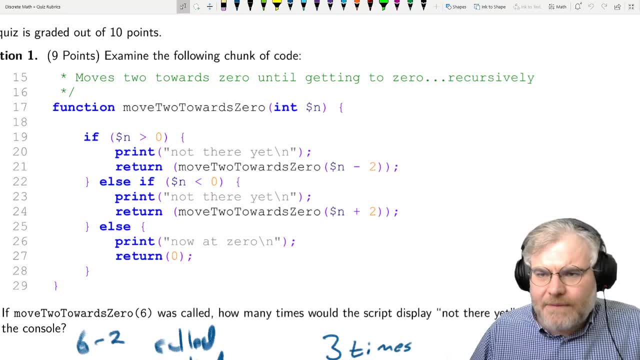 No, it's not a while loop. You can do it with a while loop, But the point is this: I'm going to do recursively, Okay. So I'm going to do this using recursion instead of using a while loop, Okay. 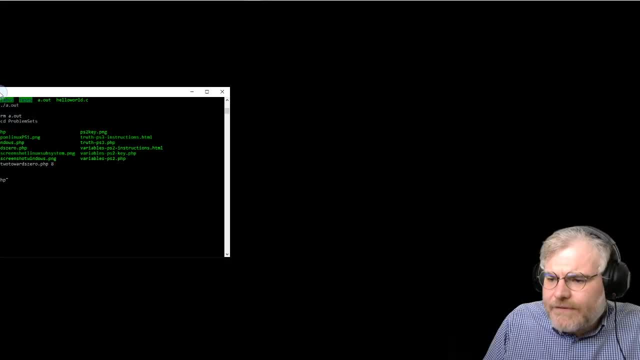 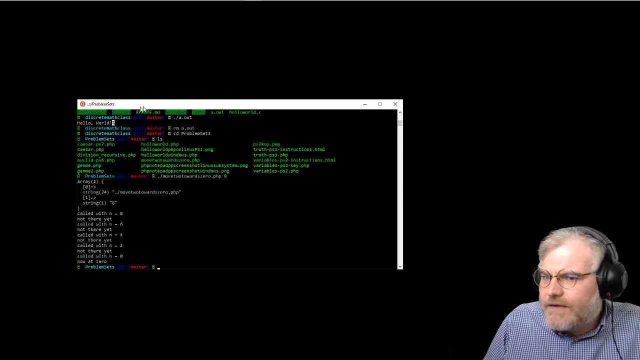 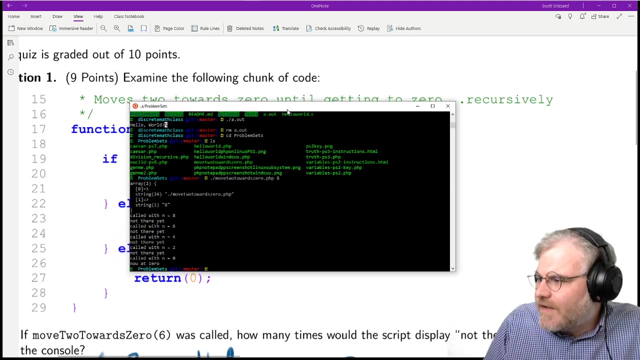 So let's see what happens. This is just an example. Let's see what happens. What happened to my screen? It's Windows. It does strange things. Why did it do that? Let's try this again. There we go. So I take this piece of code: 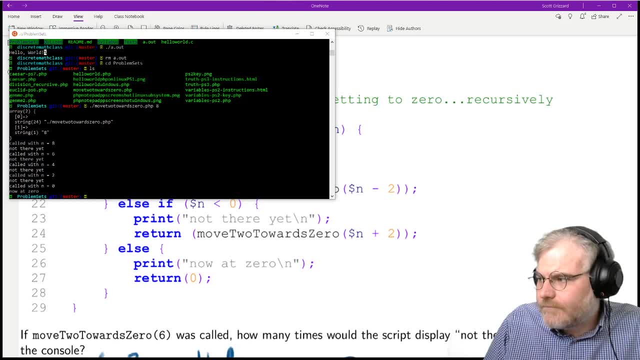 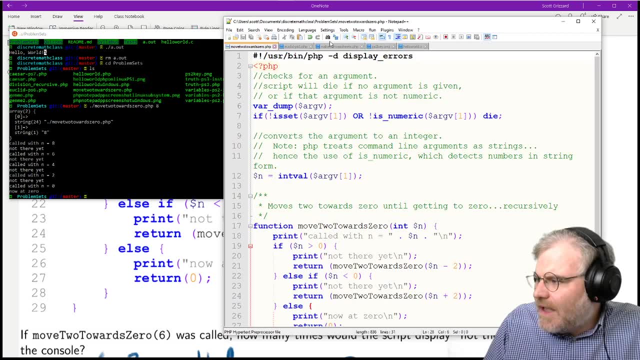 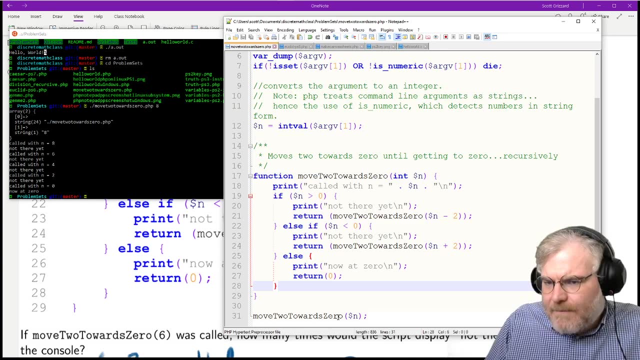 Shown here, And what I'm going to do here is right here. what I've done is I've basically added the thing so that I can add an argument. So instead of having move towards 0, 6 at the bottom here, I'm going to make it so that I have an argument. 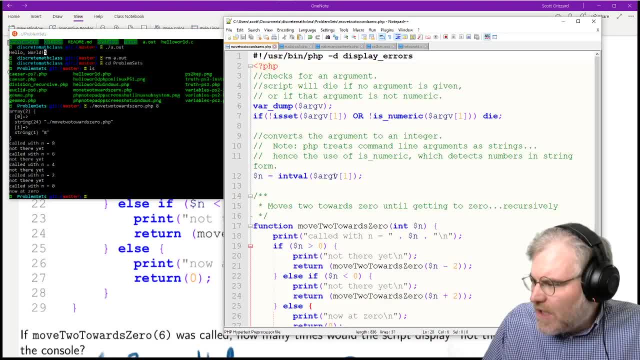 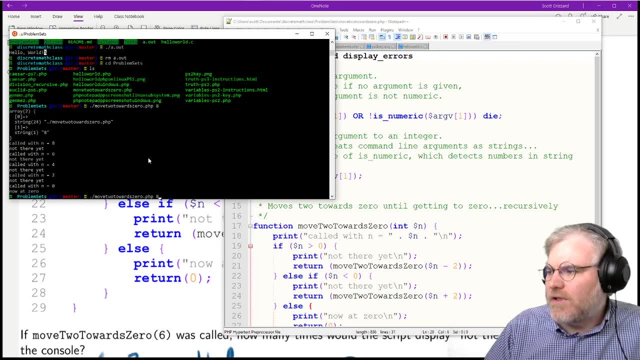 So, whatever I input is going to be the thing, And I will post this code. You can look at this code. This is very helpful in your scripts, Right? So what I'm going to do is I'm going to ask it move towards 0, 8.. 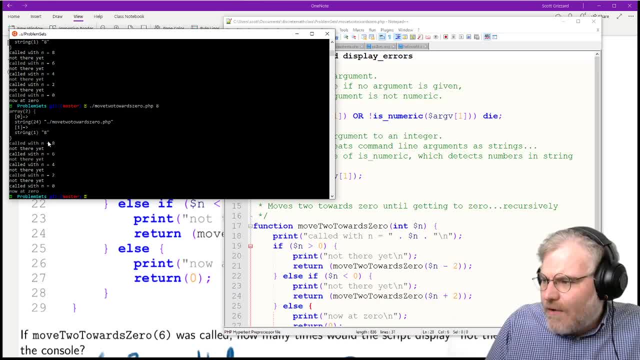 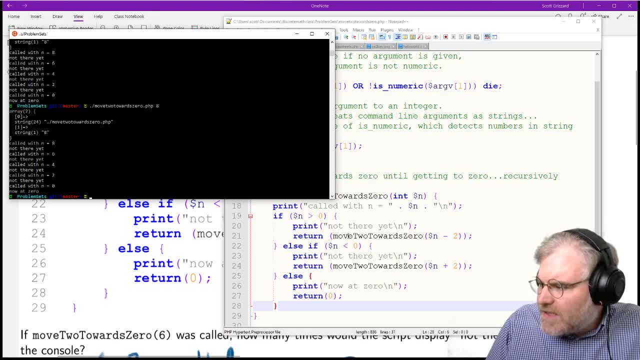 And if I execute this code, it's going to, you know, go to 8. It's going to, okay. so it starts within And it's going to call itself again, but this time with 6 and minus 2.. 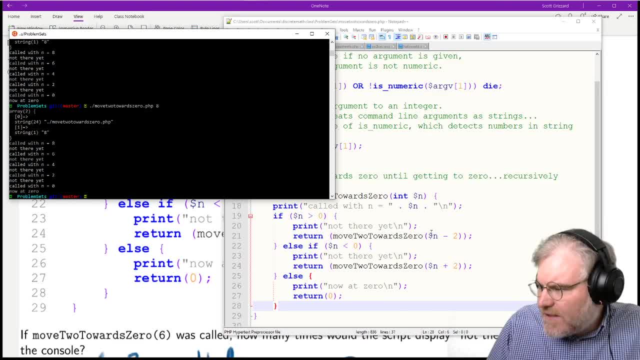 I'm not there yet It prints that And it was called with 6.. And now I'm going to call with 4.. Then I'm going to call with 2.. And then I'm going to call with 0. And when it calls with 0, it's going to say now with 0. 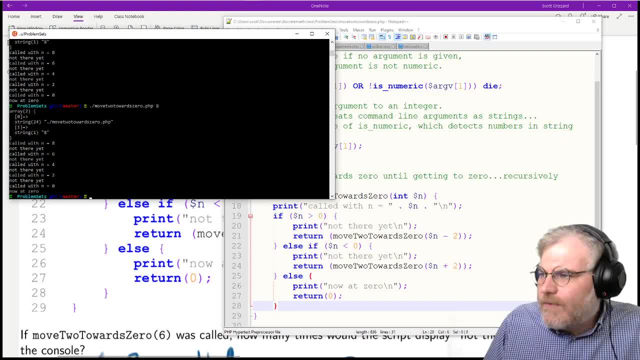 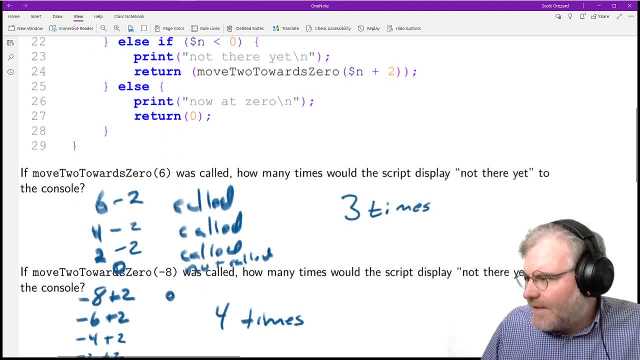 And it's going to be done. So my question was that, if I start with, I think, 6.. Let me pull back up my question. How many times would the script display not there yet? Well, it started with 6.. 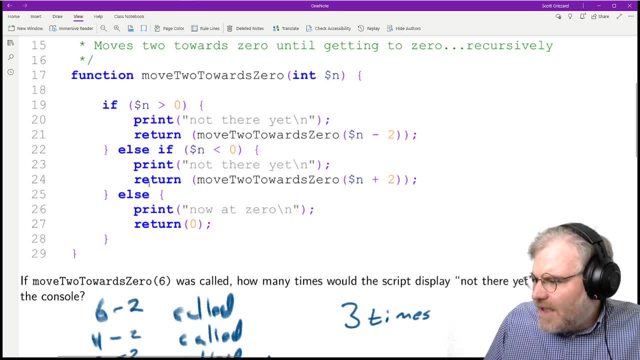 It printed not there yet and went minus 2.. Then it took 4.. It said not there yet and went minus 2.. Then it took 2, said not there yet and then subtracted 2.. And then finally it got to 0. 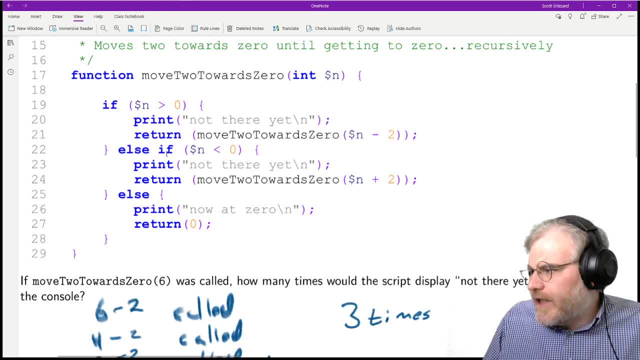 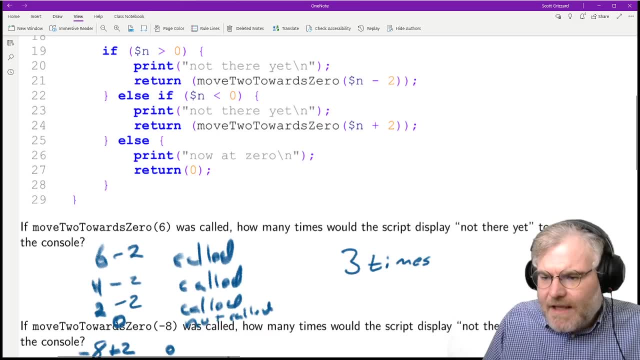 And then it was done. So how many times did it call and move towards 0? Well, 1,, 2,, 3.. How do we feel about that? 1 to 5? Okay, Of course, if I start with negative 8, it's going to be adding 2 each time. 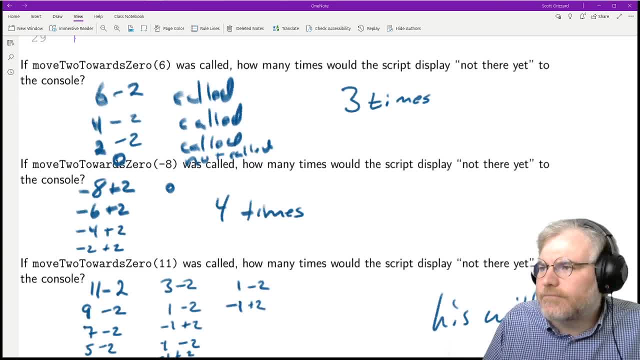 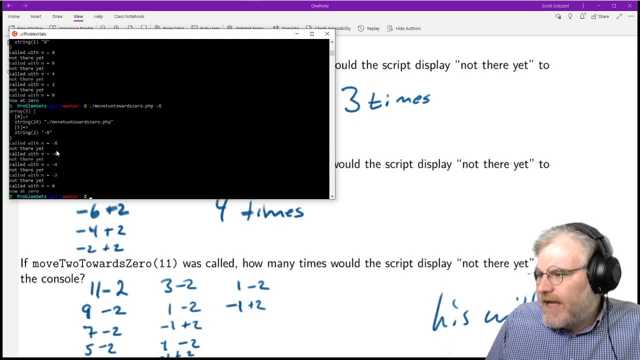 All right, So I did negative 8, negative 2.. I'm sorry. Negative 8 plus 2.. Negative 6 plus 2.. Negative 4 plus 2.. Negative 2. And so I went 4 times. 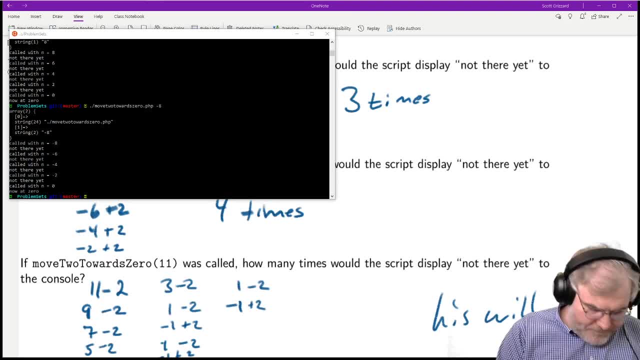 How do we feel about that one 1 to 5? So we're doing the little negative. I didn'tора sing that one because I had 2.. We're going to try this one Negative 8 to 5.. 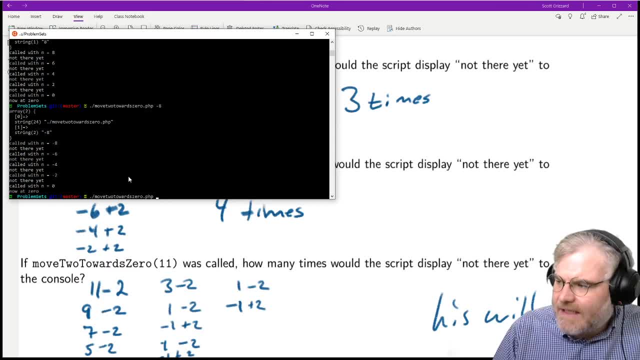 Negative 5 plus 2.. Negative 6, negative 5.. Negative 4 plus 2.. Negative: 6 plus 2.. Negative: 5 plus 2.. That's right, it's negative. I want to go down to the substitute. 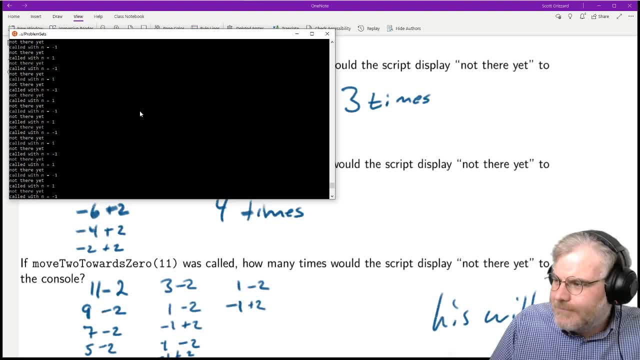 Stay on that line up here because we can just pay a little more. It does look. let's see. In order to make this stop doing this, I had to actually hit ctrl C, I had to actually terminate the command. Let's do it again, but this time I'll hit ctrl C right away and see if I can capture the beginning of the command. 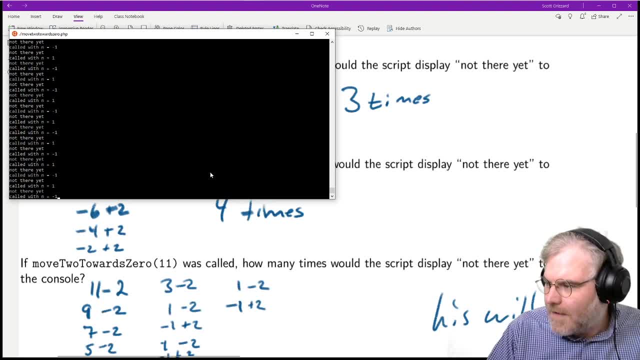 Nope, not fast enough. Way, not fast enough. let's try it again, You? Okay? well, I wanted to do the very beginning. Okay well, there's no way for me to apparently to be fast enough to do this. I would have to change the code so that it only did so many. 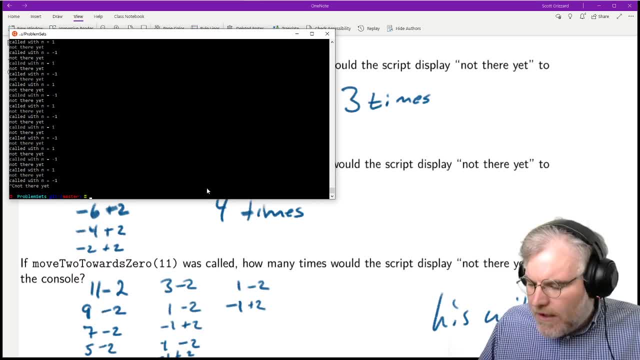 Okay, but what's the point? The point is that it goes 11, 9, 7, 5, 3, 1, and then it goes to negative 1, and then it goes to positive 1, and then it goes to negative 1, and then it. 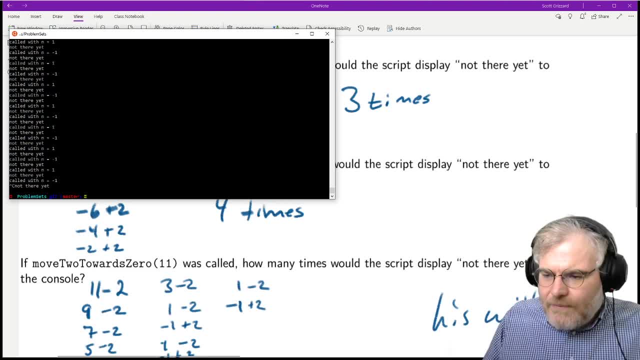 Goes to positive 1 and it never stops. So how do we feel about this? that it would never stop? 1 to 5?? All right, it's stuck in an infinite loop. Okay, and remember, when I say the word never stops, I mean I mean that you know, if we left this thing running till the end of the universe, it would still be going. 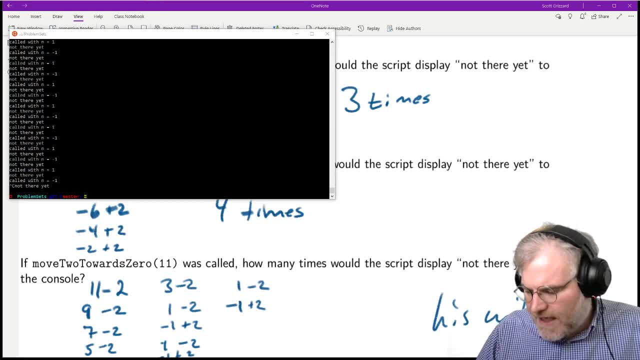 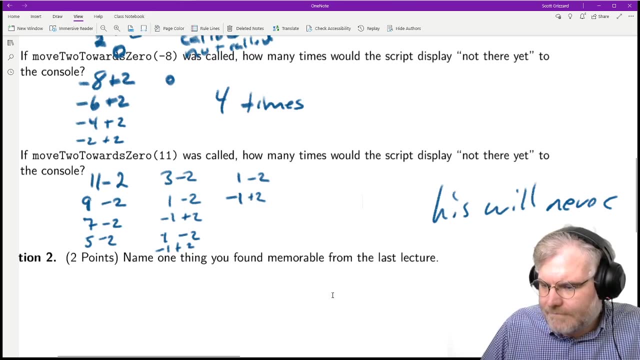 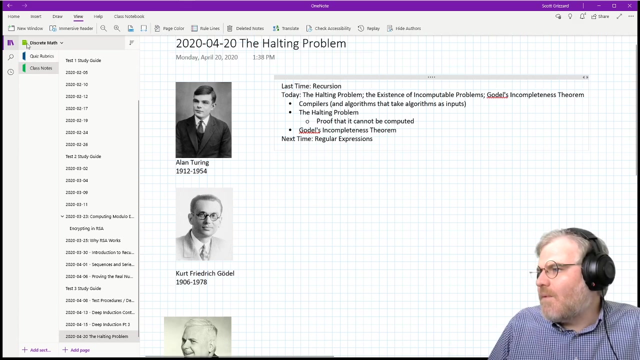 All right. When I say never, I mean it in a very strong sense. Okay, Are there any questions about this problem? Okay, so that was the big idea behind recursion. so the question is: why do I care? Let's go over it. so today, what we want to go over is something called the halting problem, and 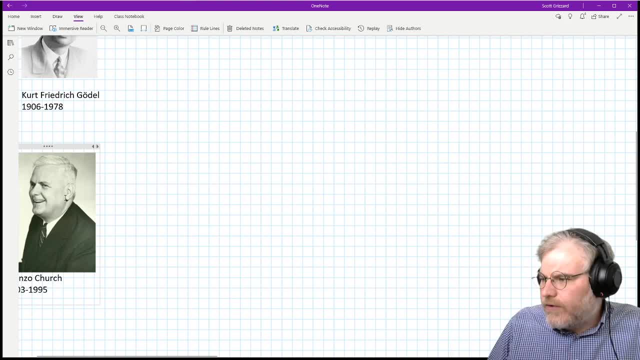 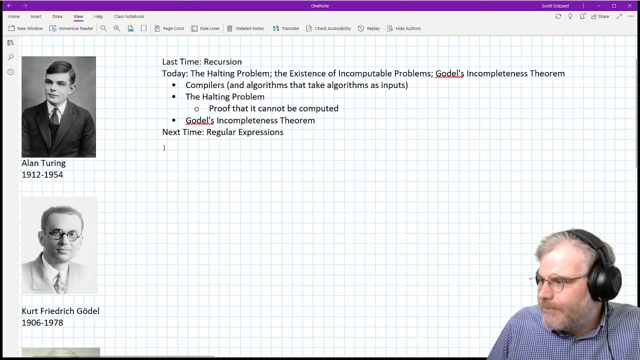 These are the three big giant. I've got Turing Godel and Church Church. for some reason his picture is not Going to cooperate and put his dates where they should be. Not that Church is smaller than these other two, but you know, let's just make it light up. 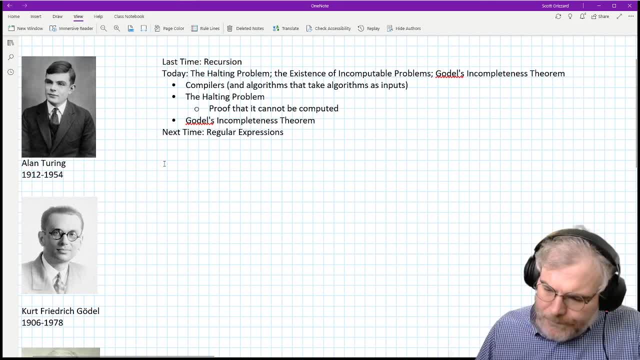 Okay, so we got Turing Godel and Kirk Church, and In order to talk about this problem, we need to talk about a compartment. a compiler is so when I think about functions And, by the way, if your head does not hurt, at the end of this, 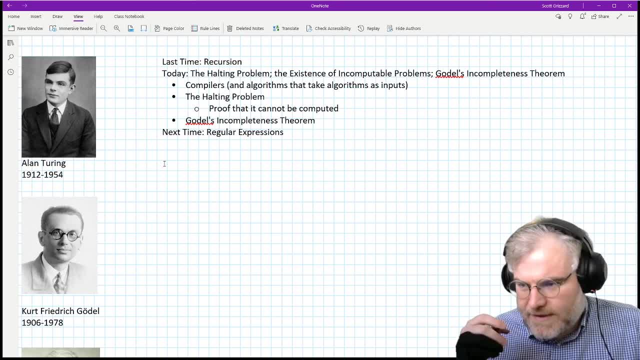 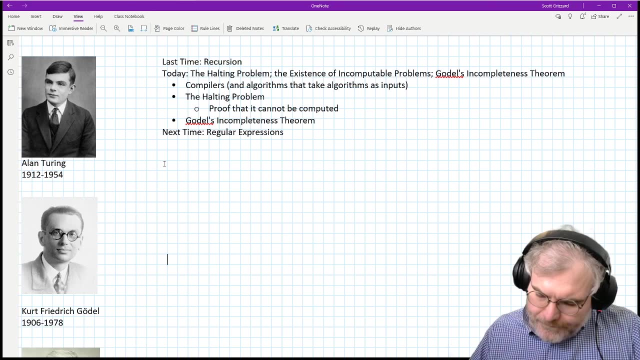 thing. Okay, then you didn't listen well enough and you need to rewatch it because your head should hurt while you're doing this. Okay, this is weird. It's important, but it's weird. Okay, so what's a compiler? Anyone have a good definition of a compiler for me? 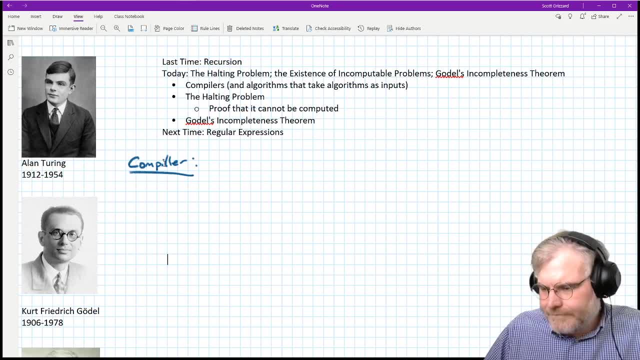 Or just a so-so good definition of compiler Right. It's a program that translates algorithm. Did I spell it? Oh, yes, one, No, I Did spell it right in the when I said it before. I'm not in the computer science department and I'm really not in the English department. 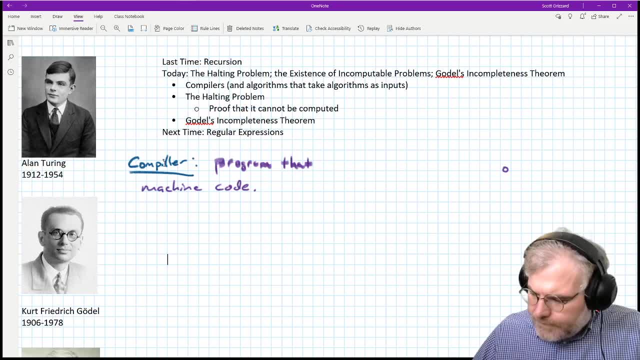 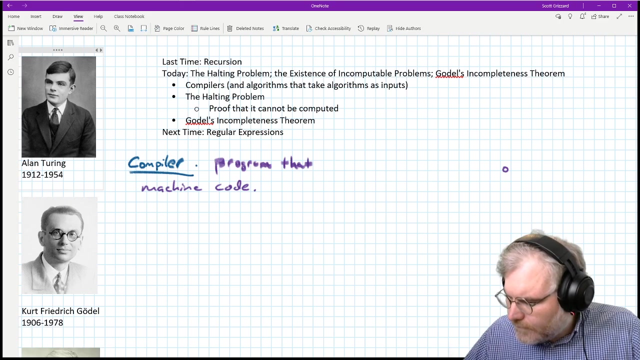 It's a program that Translates Algorithms And to machine code. For our purposes, that's enough. I Don't know what this thing is doing. It was doing this before. Okay, It's back. If this thing keeps happening, what's going to happen is I'm going to have to 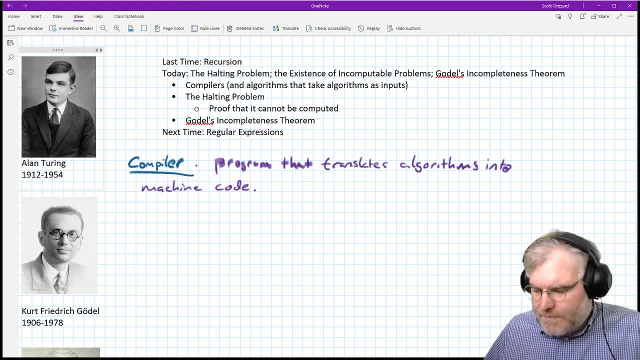 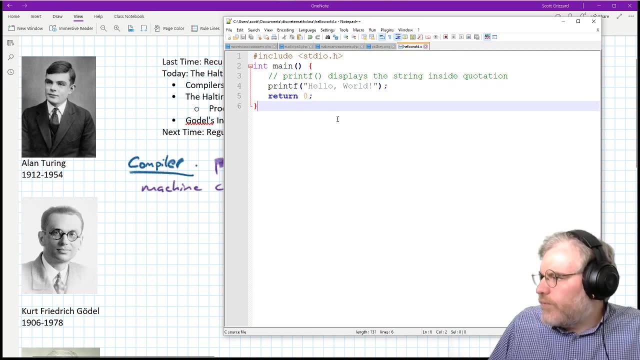 Wing it on the thing, because this is, this was happening this morning and it's getting worse now. Anyway, So the important. so let's give an example, right? So, GCC, I've got the cease compiler, compiler. So here's hello world written in C. Is everyone on board with this? This is the C. 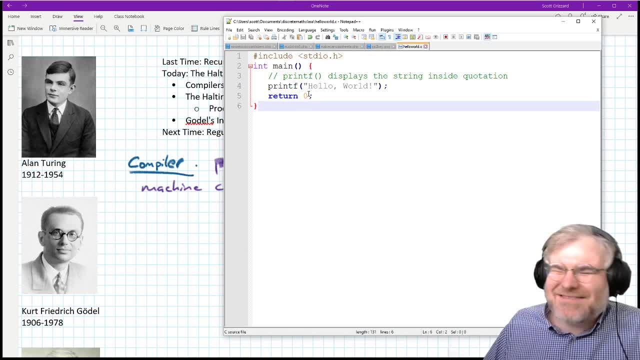 Now, PHP is not a compiled language, Neither well Java can be or can't be. Java compiles into something called bytecode, which then has an interpreter, or a virtual machine that runs on it, which is basically an interpreter, Or you can compile it in the machine code using a Java. 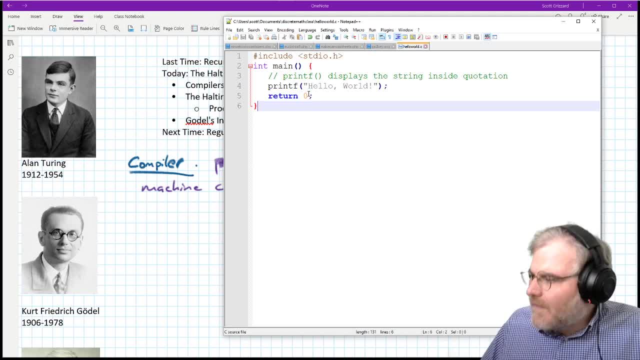 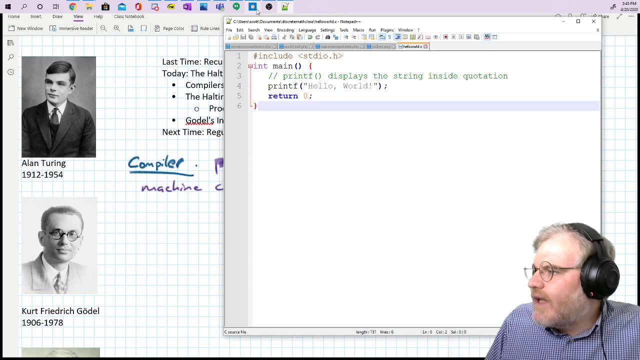 compiler as opposed to the bytecode compiler. But C is kind of the standard code thing that I compile with. So let's take this lovely little program here. This is machine out. Now, the computer can't run this straight, It doesn't have. well, it could if it had an interpreter. 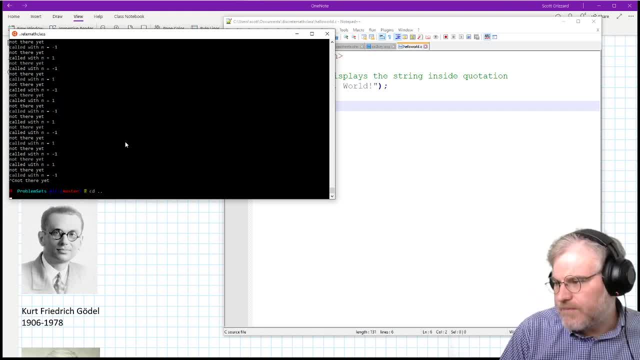 but it's not meant to be. It's not like PHP which is meant to do this. So there's hello world CC. So I start up GCC and I do hello world dot C and I hit enter And then when I hit LS again, 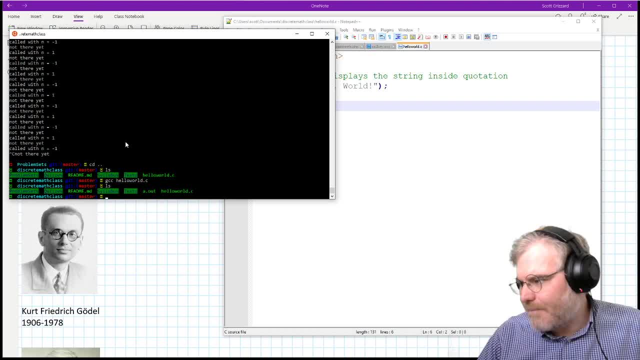 I get this A dot out because I didn't specify what I wanted my output file to be. It just did A dot out. So now, however, I run this as a program and this is actually in machine code. So if I do less A dot out, right, it's going to give me gobbledygook. 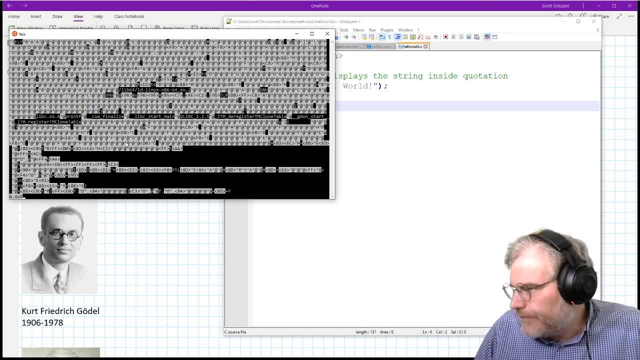 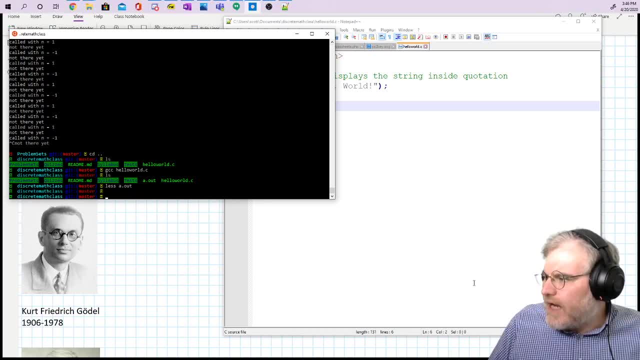 because it's not going to run. It's not text, It's machine code. All right, Are we all on board with this? So what this program did was it took my text and it created machine code. And so if I do this, but if I run the program, 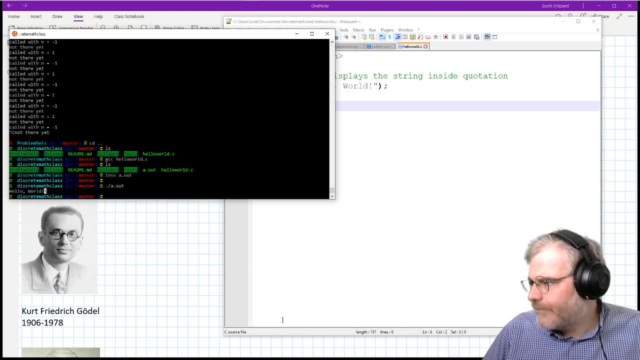 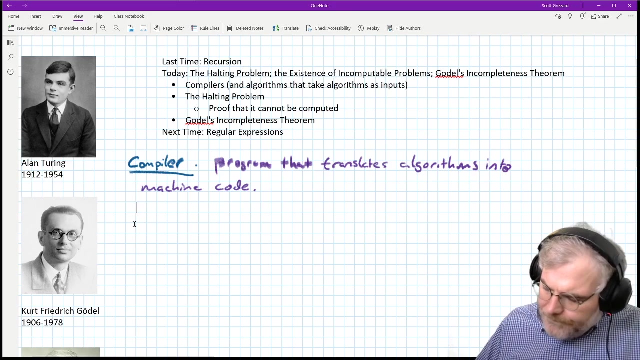 I get what I wanted. Hello world, Okay. So how do we feel about what a compiler does? How do we feel about what a compiler does? I get gobbledygook, Okay. Now here's the important bit. The important thing is that I can compile my compiler. 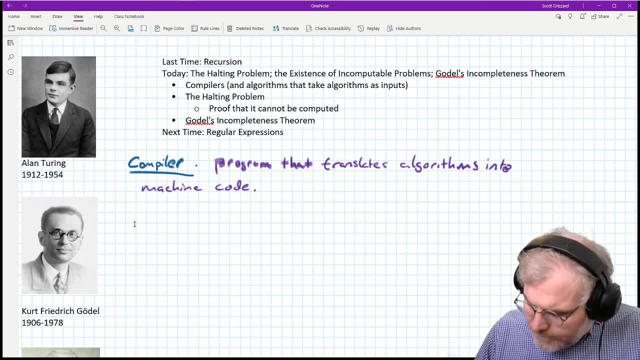 All right, So what I need to do is: You want to call it a compiler? Yeah, You want to call it a compiler? Yeah, Okay, Okay, How do I do all that? You can do this, So here's the compiler. 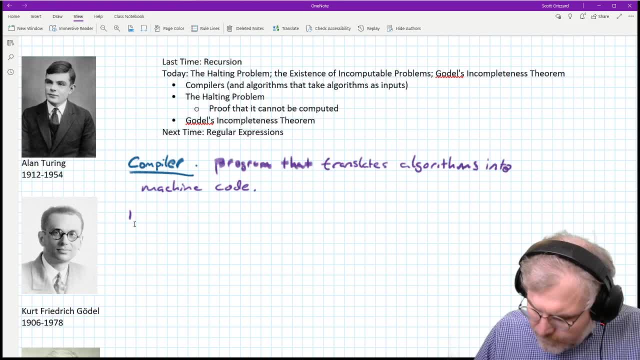 All right. So now I know what the compiler does. I can write my code here on my computer. I see, I see, I see. Now in this example I'm going to write a compiler that doesn't have a computer. 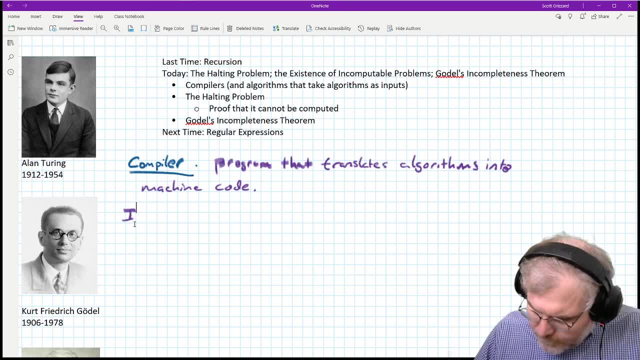 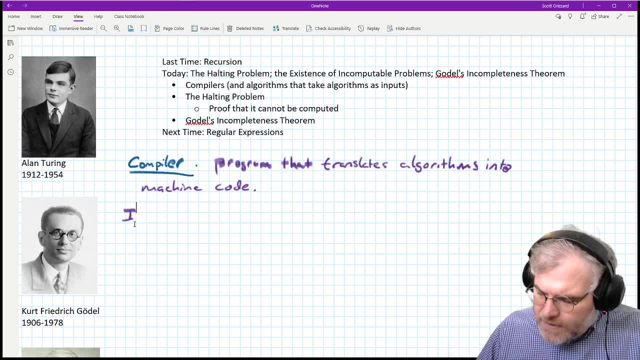 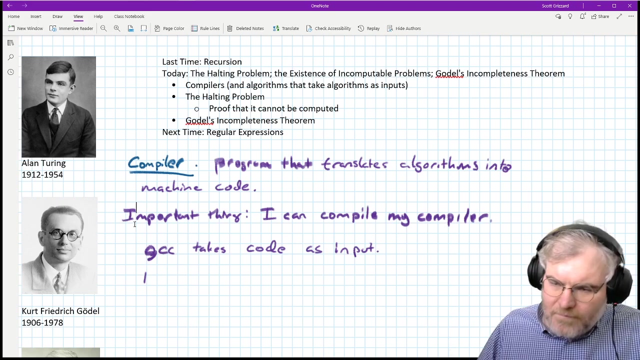 Here's my compiler, C++. I'm sorry, the GCC takes code as input. It can take its own code as input. In other words, I can run GCC of GCC, okay, and this is called self-hosting, Okay. How do we feel about that? one to five. 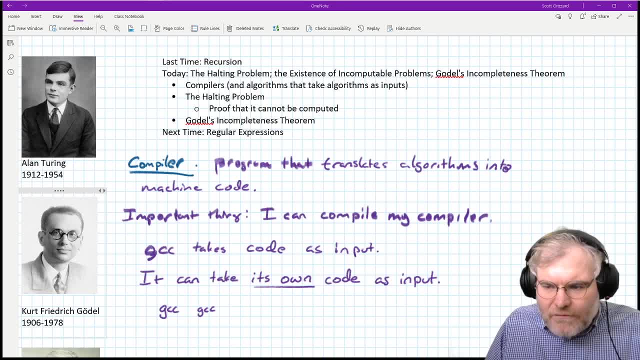 This idea that this function can call itself the algorithm for itself. right, This function can take the function not as its own input. So in other words, I take GCC, the code for it written in C, and I compile it using GCC. 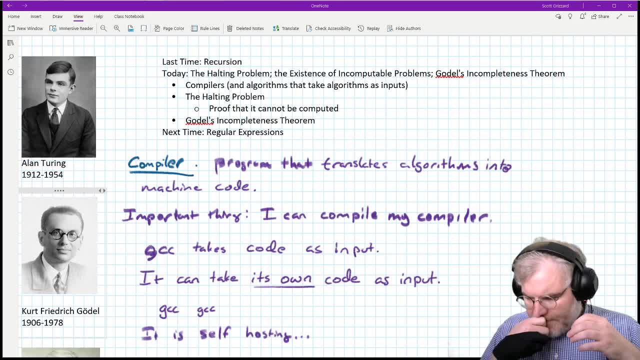 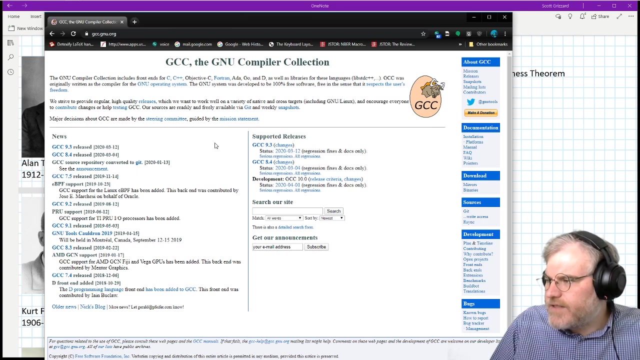 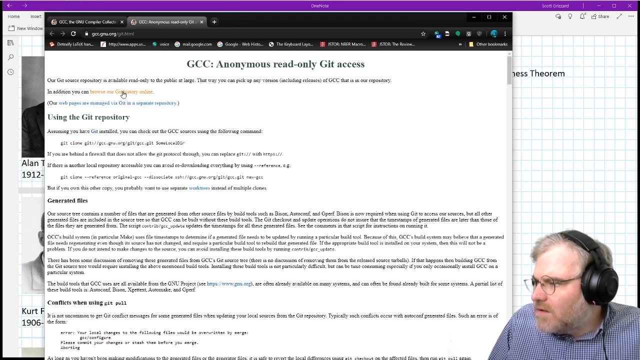 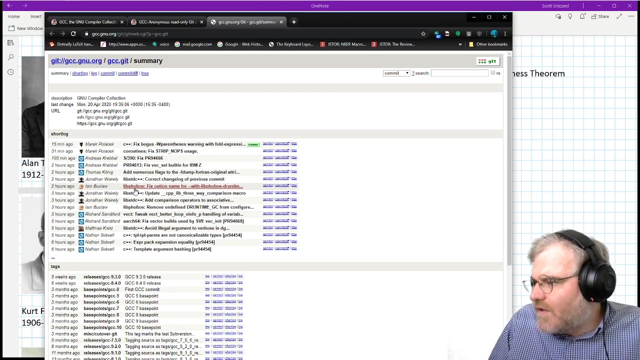 Okay, And that's also what it generalize. sorry, the GNU C compiler: Okay, this thing, right, it is its own compiler. okay, and if you want to, you can actually look at it. so if i go to git, so this is the gnu's git, okay, and i can actually see the source code. 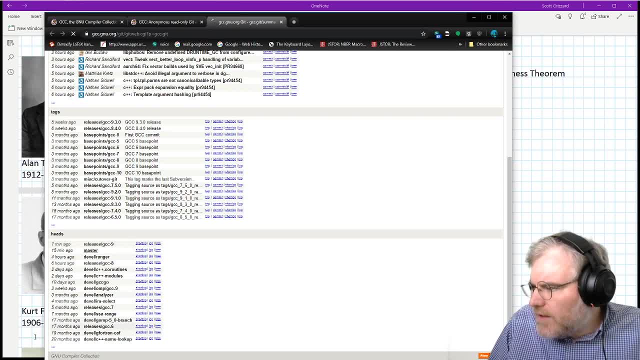 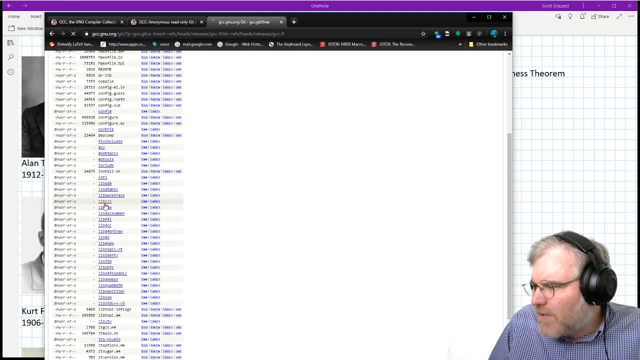 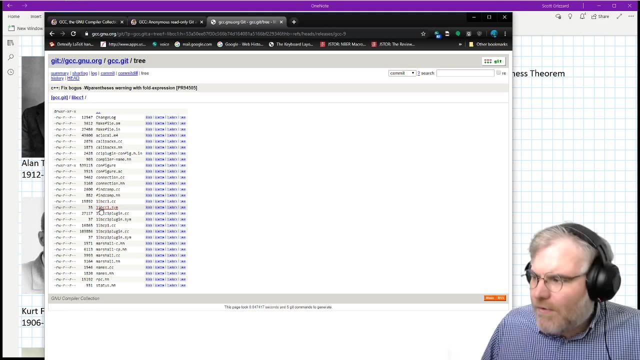 so let's see, here's the tree. i've got all the permissions that go into it, and then i've got all of these little libraries right: libcc. these are all written. these are header files, but the point is that the program itself is written in c, along with some other things, but it's mostly written in c. you know, it's got some assembly. 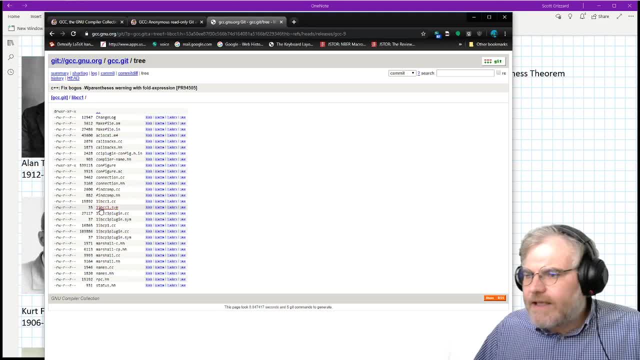 in there and stuff like that. um and it, it can be used to compile itself. so i compile a version of gnu cc and then i use that version to compile the next version. but at some point, right, i can also just use it to call itself. so, for instance, i want to compile a new linux kernel. 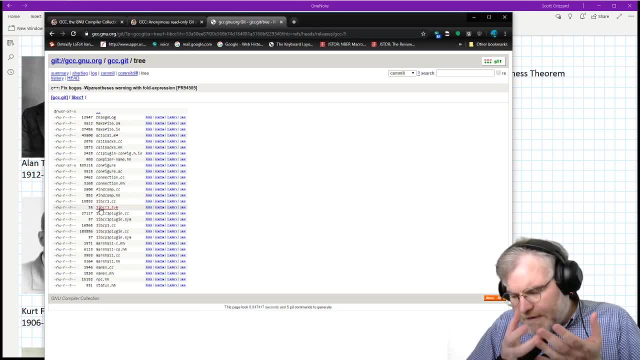 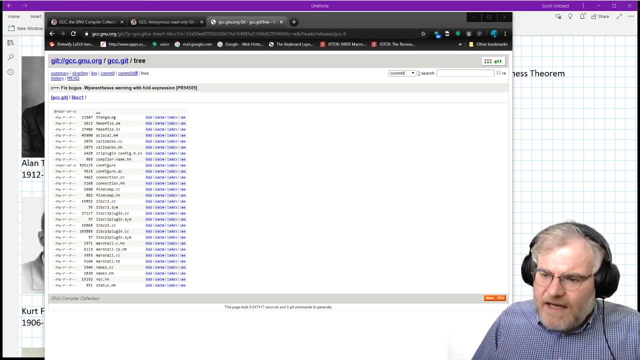 i can use linux and gcc running on top of linux to compile a new linux kernel. in other words, it's self-hosting. i can call gcc on gcc itself- okay, and that's weird. okay, and gcc running on top of linux. c stands for the gnu c compiler. 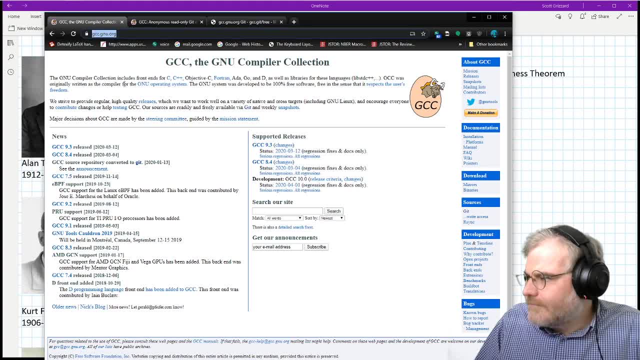 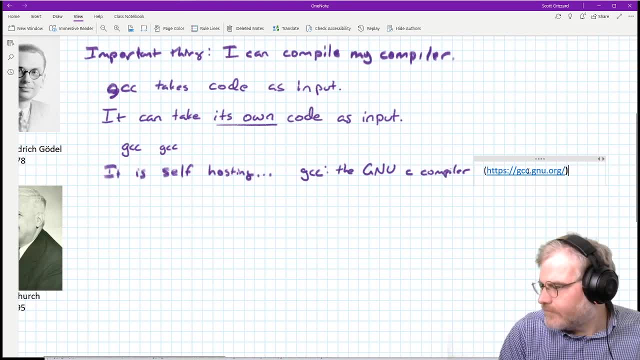 okay. so how do we feel one to five about this idea that i can, that a function can call its own code? in a sense, there exists functions like compilers that can call themselves, that can accept themselves as input, right, so i usually think of a function as taking something as input, and that function can be. this is different from. 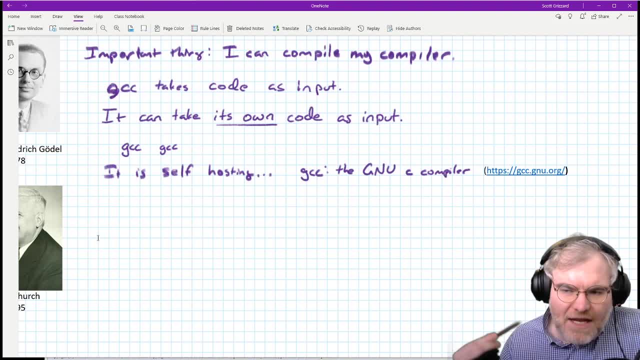 a recursive function which kept calling itself. now, now i'm calling myself as the data. okay, my input for the function is the data. how do we feel about that? one to five? i'm not. this is not recursion, yet all i'm saying is that i can, i can, i can this idea that a function can call itself as data. 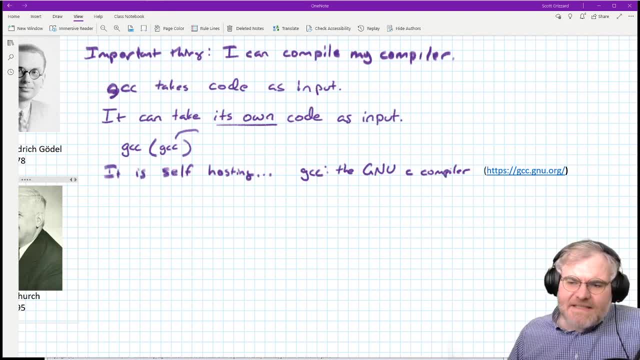 um, and you see this a lot in the in in java when you do certain types of injections, um, and in javascript it's all over. ecma script, oh my goodness, where you have procedures and then you have them call other procedures as input. so it's a little weird, this idea: php sort of supports. 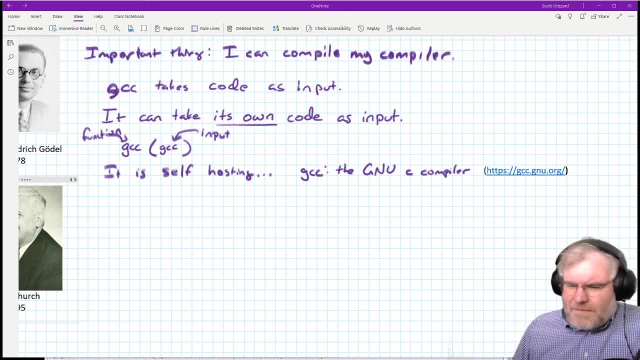 it, but not really okay. so what does this have to do with the halting problem? you see, this is the theorem, theorem this is uh, tuering godol church, a bunch of other people, um, so this, whether or not which one's the problem, right, it depends which version of the theorem you 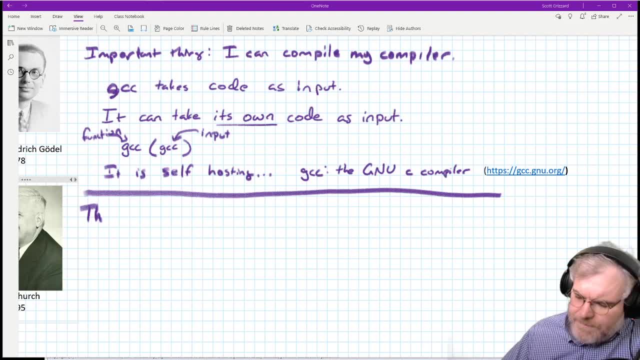 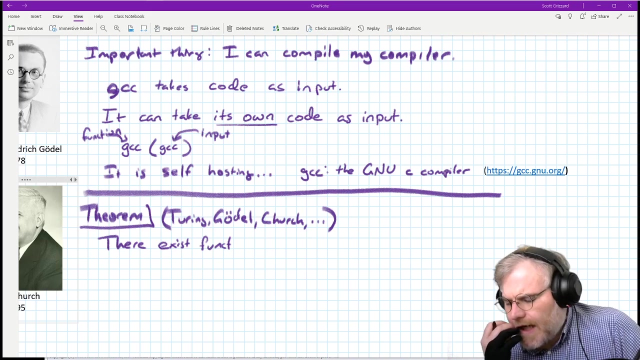 call it. There exist problems that are uncomputable. Okay that I can't write algorithms to do. Okay, Proof, Okay, so we'll do this as another theorem: The halting problem. Let's just say here The halting problem. 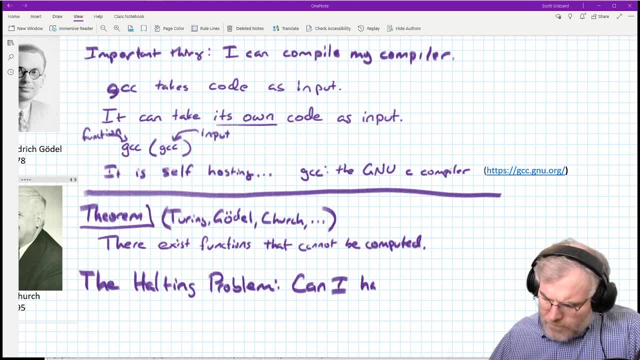 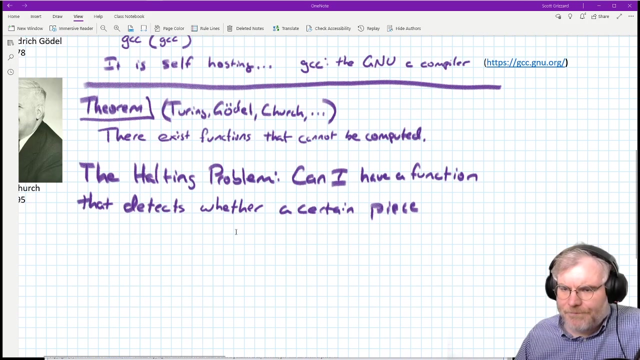 Okay, so can I have a general function that detects whether a certain piece of code, given a certain piece of code, is a piece of data with halt? Okay, that's the halting problem Now. for example, today during on the quiz. 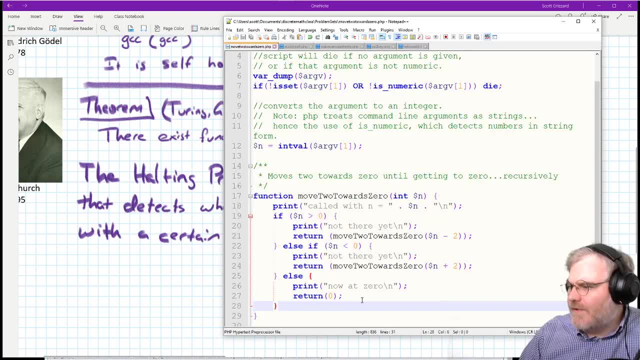 you had this problem here. right Here was your algorithm, right. This moved towards zero. Now, if I gave this moves to zero, if I fed the algorithm moves to zero, for the function would halt, Whereas if I fed it any odd. 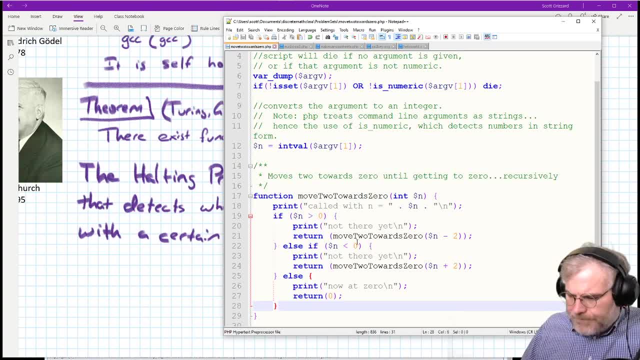 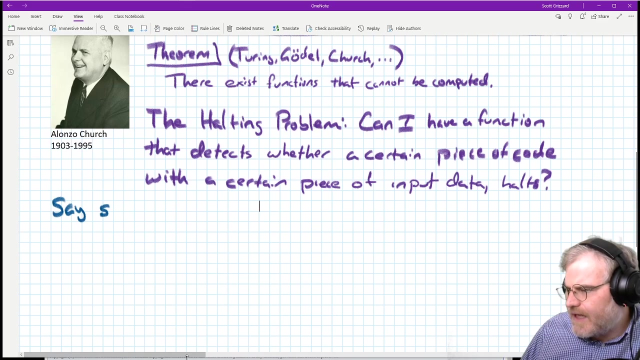 any odd number, the function would not okay. So let's say that this function exists. I would call it check halt. Okay, so let's suppose that such a function did exist And I call it check halt. Now the thing's struggling to keep up. 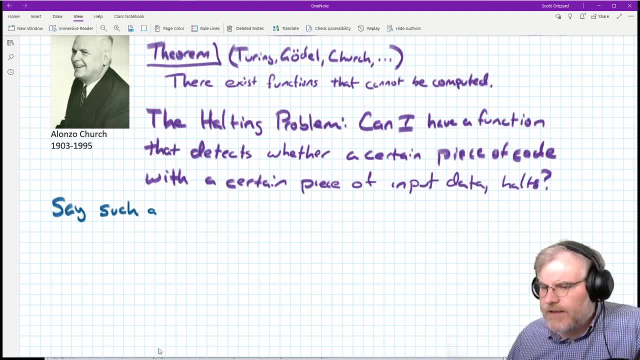 And I'm sorry about the lag, But the internet. I'm looking at the bars right now and it's going And there's nothing I can do. Okay, So well I can, except that if I do it now it's gonna cause the whole thing to freeze. 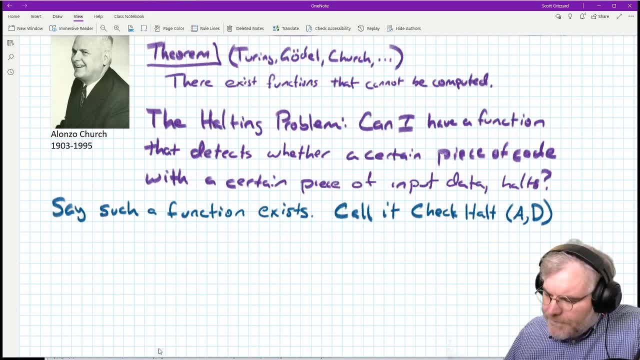 by the time I'm done. All right, Okay, So now if I fed this function, this function, I'm gonna go back and I'm gonna go to check and I'm gonna load up all of my values I have. 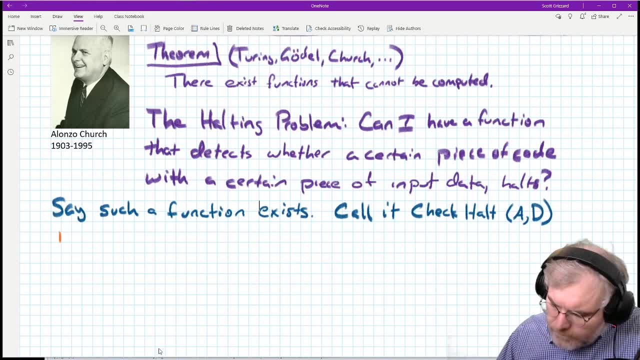 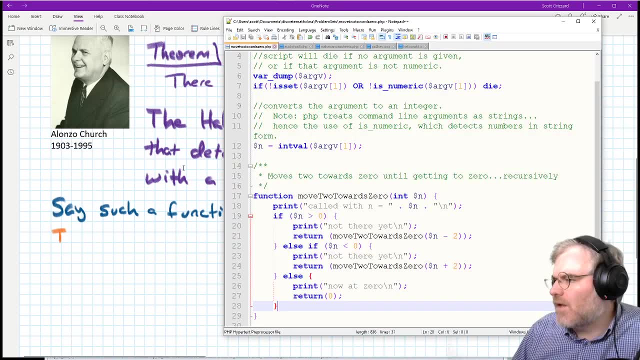 So if I ran check and I changed the down value to zero and then I moved it to zero, that's gonna lower the value. So I'm gonna type in the passcode of zero and then I'm gonna export this data. 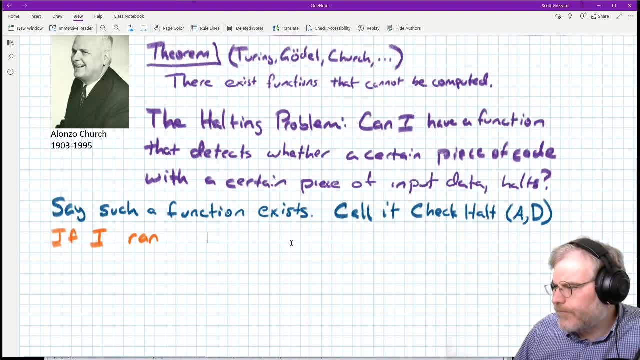 and then any part of the data that I have to run. I'm gonna print out the data And that's what that means. As you said, I change the value of my data. I change the value of my data. Is it going to sync check halt for me, or did I just mess it up by writing on this one? 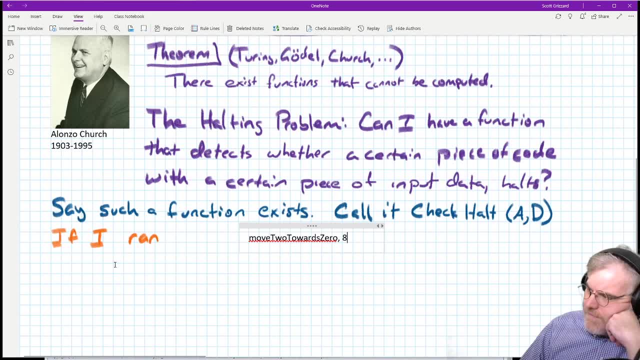 and that one at the same time. Only time will tell: Let's hold on. Ah, there it goes. So if I run, check, halt and move towards 08,, what's it going to return? 08. 08. 08.. 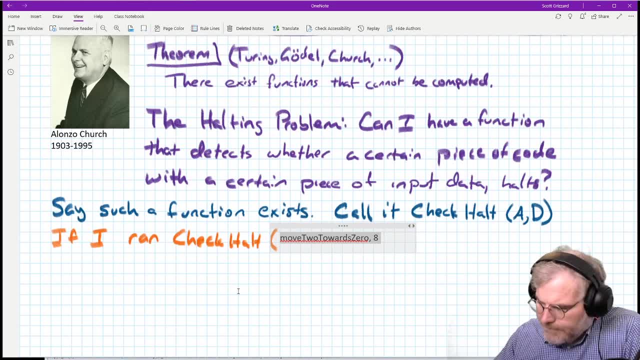 08. 08. 08. Okay, so this algorithm- excuse me, it's thinking about working. It's still thinking about working. Okay, it's not working. Okay, so it returns true if algorithm A hearts with data D and false otherwise. 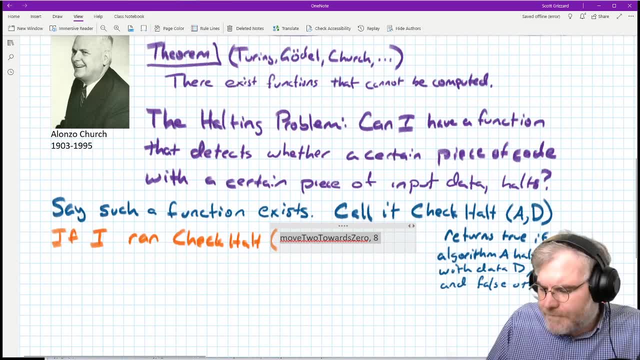 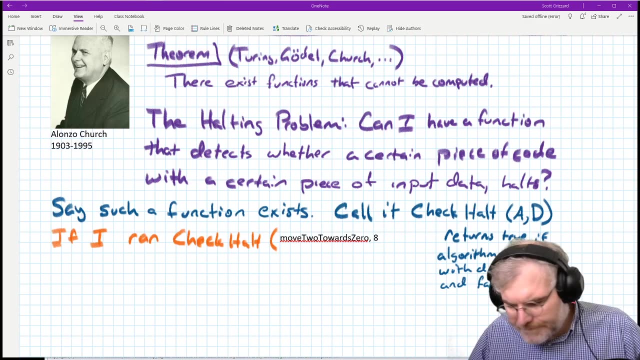 All right, is everyone on board with what this function does? So 1 to 5.. Oops, let's move towards 0.. So 1 to 5, how do we feel about what this function does If it existed? It reads the algorithm. it reads the input data. 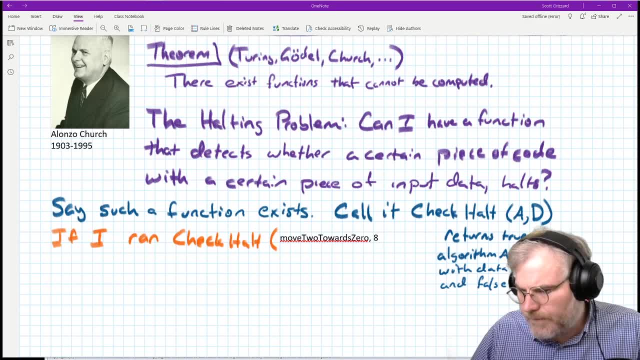 and tells me whether or not I'm going to wind up in an infinite loop. And now it's got two 8s there. It's still returning the same thing. I don't know why it decided two 8s was appropriate, But it did. 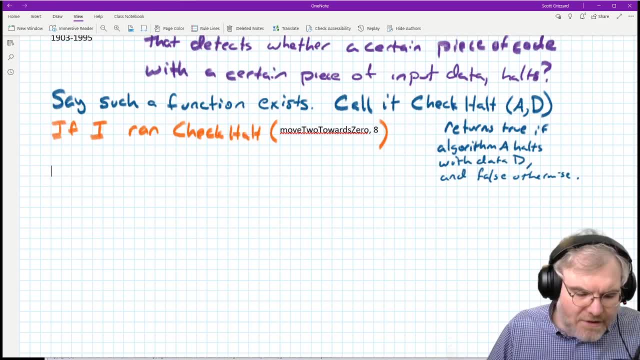 Okay, So if I ran it with that data- sorry, I just hit the mic with my phone, with my hand If I ran it with that data. So check, halt. We've returned true, whereas if I gave it an odd number. 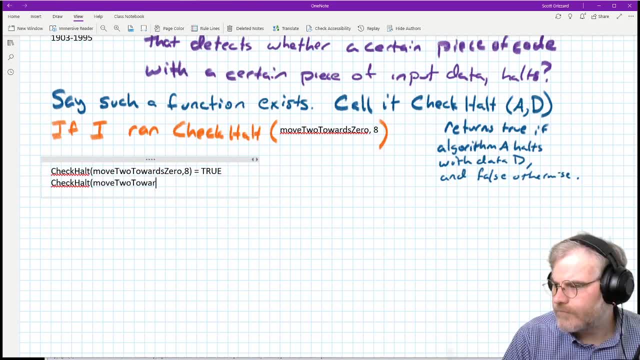 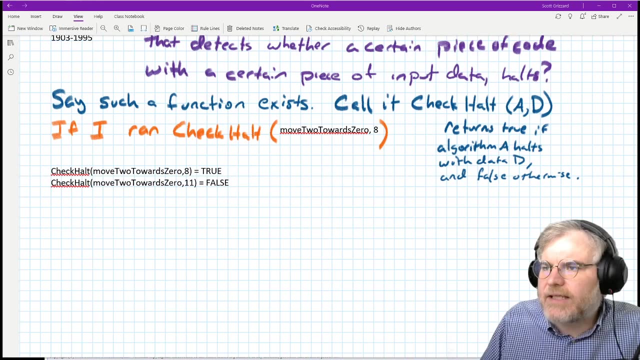 okay. so how do we feel about that? right, if I ran it with one thing I'd get. if I ran it with an even number, I wind up with true, and if I run it with an odd number, I run up with false, because if I give it an odd number, it's never gonna. 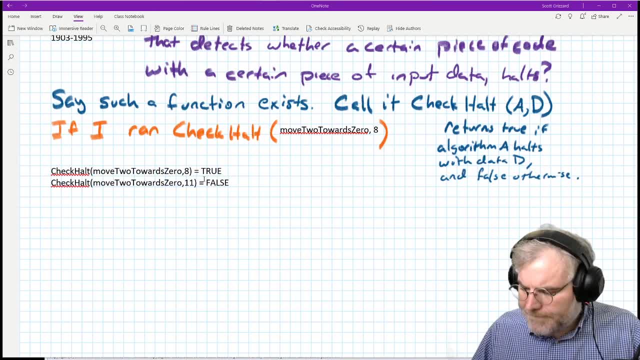 hold. okay, okay, all right, okay. so let's suppose such a function exists here. it's still failing. all right, let's go to Plan B here, and Plan B will necessitate the use of Plan C at some point, because the internet's stupid. right now I need OBS, OBS, OBS, OBS. 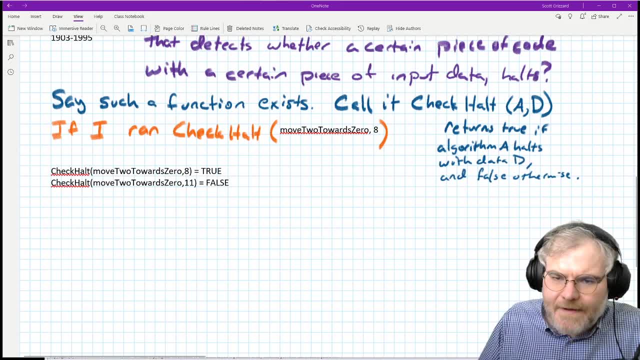 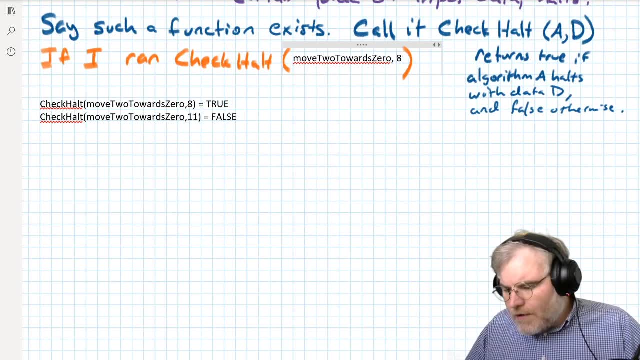 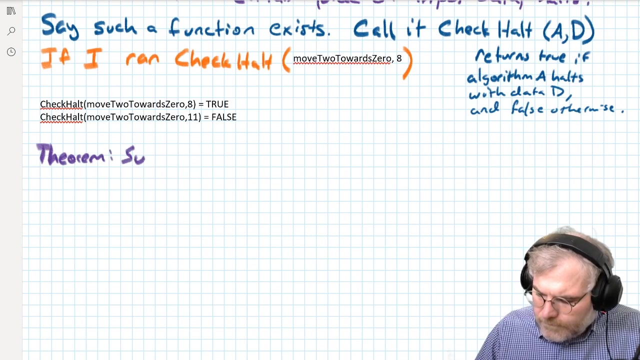 all right, let's see if I can make it work this way. okay, so, okay, you, you suppose otherwise. suppose such a function does exist, okay now, well, if such a function did exist, right, and remember, this check function takes as its input an algorithm and a piece of data. that's the data that goes in: an algorithm and a piece of data. 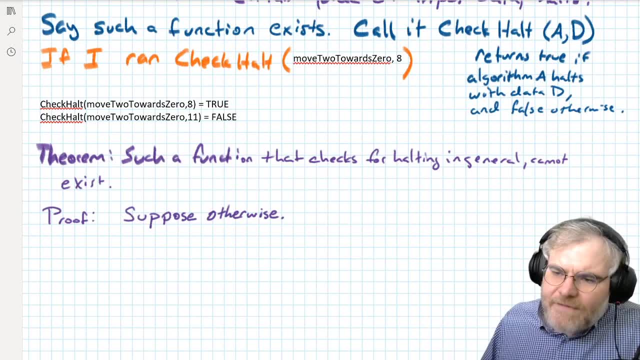 okay. so how do we feel about what's happened so far? one to five? um, again, it's not so. how do we? oops, come on, how do we feel about this? one to five, okay, I'm going to suppose that such a function does exist. okay, now I'm going. 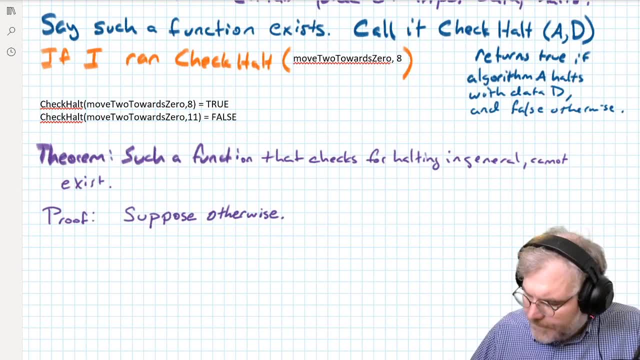 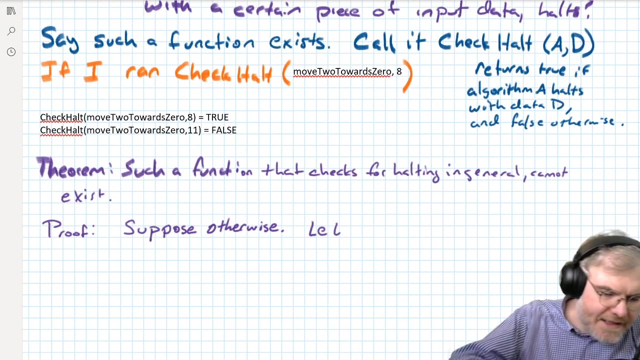 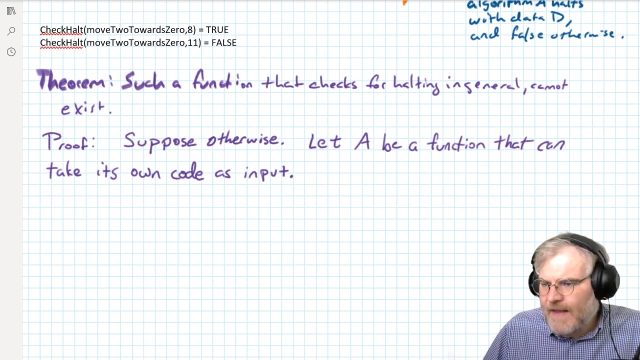 to be. let a be a function. okay, it's now, it's not letting me write anymore. let a be a function that's kind of like a compiler. let a be a function that could take its own code as input. okay, how do we feel about that? so, how do we feel about that? okay, I've taken a. 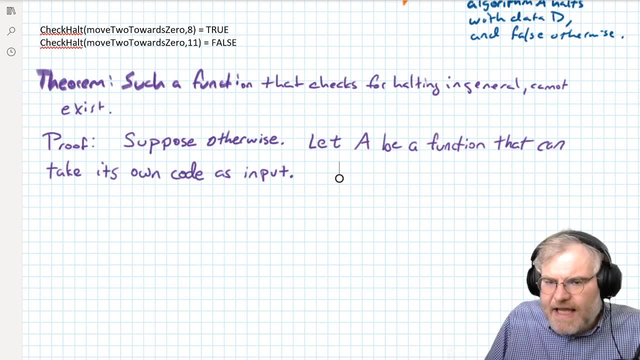 function that's like a compiler and used it. and you know, I've taken some function that looks like a compiler, something that could take its own code as input, an algorithm that could take itself as input. okay, and now I'm going to run check, halt AA. right now I can run. 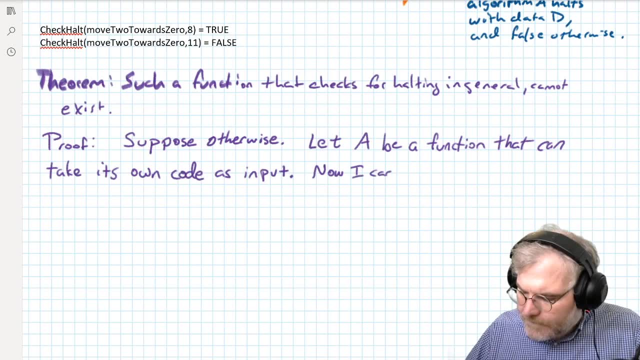 ***, ***, *** *** ***. And it will return true if A would. it returns true if A would halt given A. I love this. Every time it fails to write. I sit here doing this, right, I'm like I shake the pen like it's ink, right. 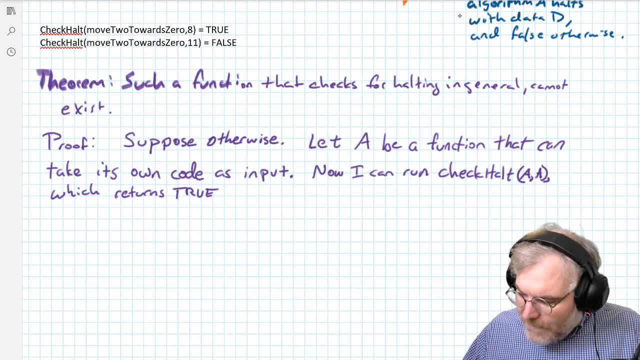 Come on, Marie. No, It's not going to work that way. Returns true: if A of A falls, It falls otherwise. So how do we feel about that little bit of setup? one to five? Okay, All right, All right. 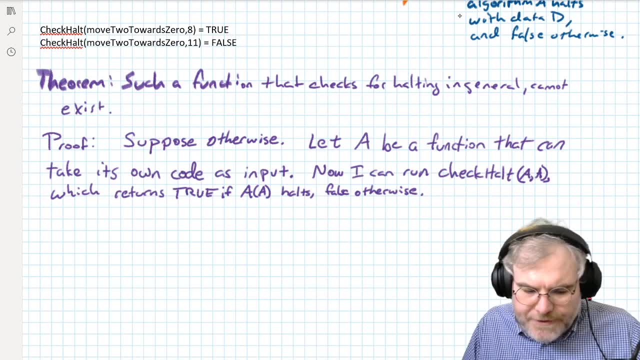 Well, now I'm going to create a new function And your book calls it test, so I will call it test, And test does as follows: Normally in the literature it's called G. Your book decided to call it test. I don't know why, but we're going to call it test. 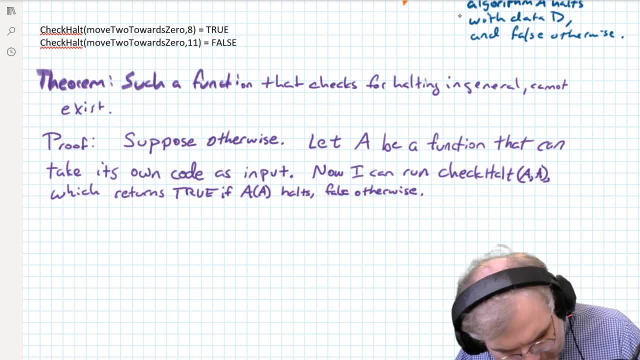 And test does the following. Test looks like this: Where did I write it down, DDDD? So now I'm going to create a new function. Where did I write this function? I'm going to create a new algorithm. Test Is the following algorithm: 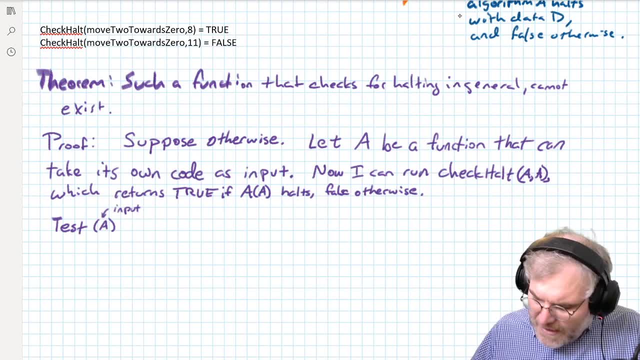 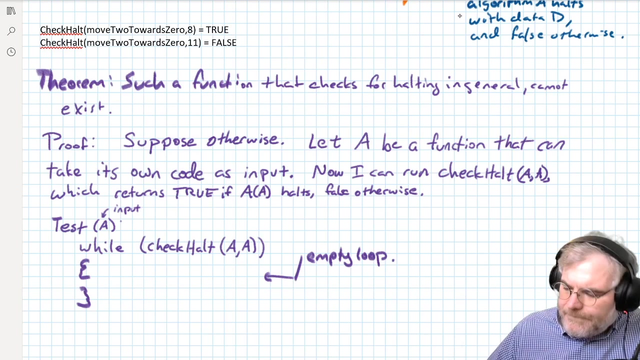 So test takes algorithms as input and it looks like the following pastry: Dd A, Dd, b, a, ah, c, V, I, a. I'm going to emphasize that Empty loop. Okay, And that's test. 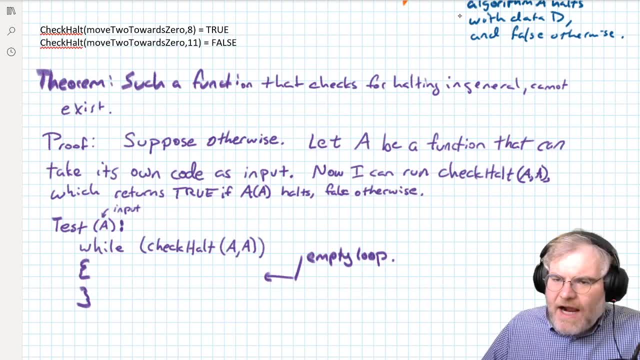 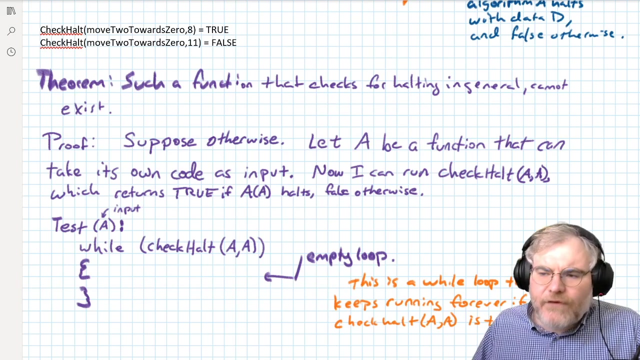 Test is nothing but an empty loop. It's a while loop that keeps running. So how do we feel about that piece of this? 1 to 5?? This is the idea that what I've written is a new function that will keep running forever. 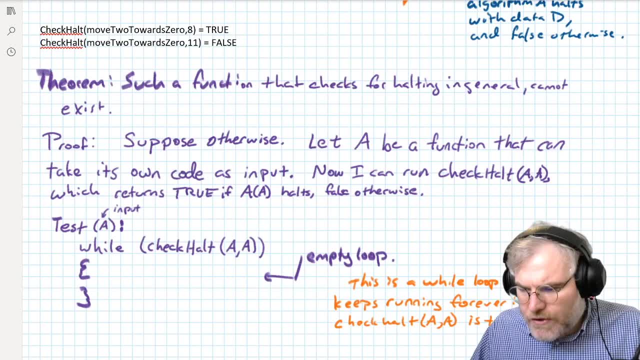 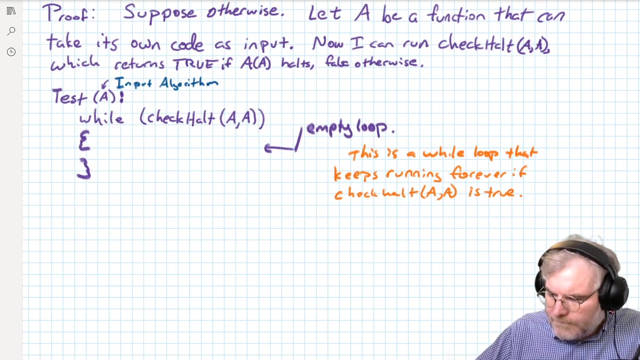 as long as check halt returns true, Right. So if check halt AA returns true test, runs it Infinite loop. Okay, So it's going to input an algorithm as it's input. Now I'm going to run test of test. Okay. 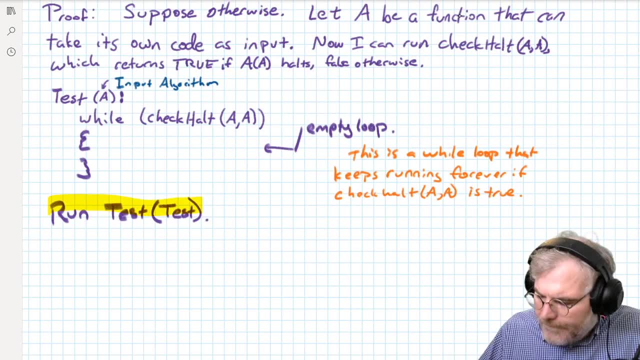 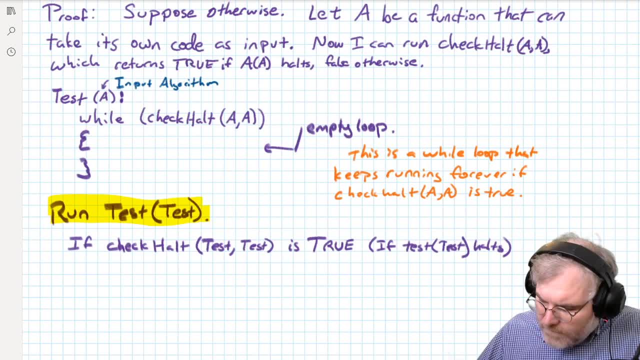 If test test halts, then what does test do? If test test halts, then what does test do? If test test halts, then what does test do? So if this thing runs forever, then what does test do? That implies: 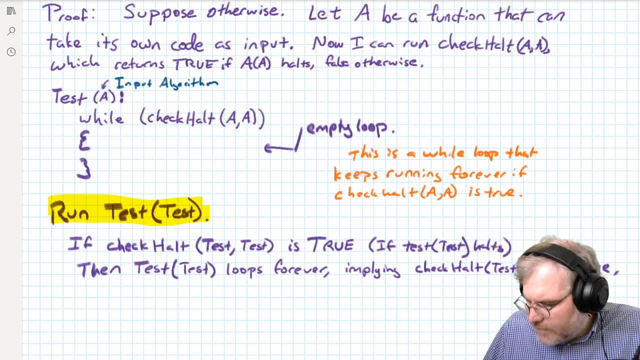 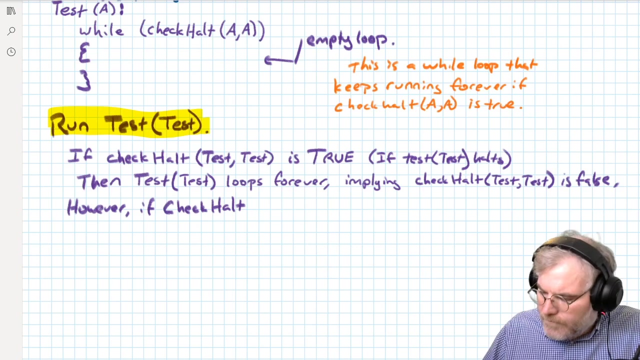 then what does test do? That implies that test test was false and it halted. However, if check halt is on it now, Just let me think about it. Let me look at my schedules. Okay, Just look at my schedules. 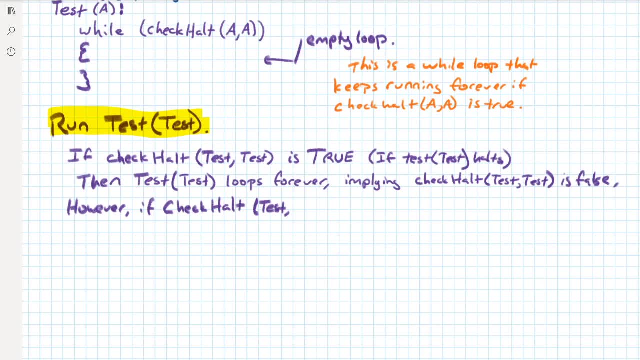 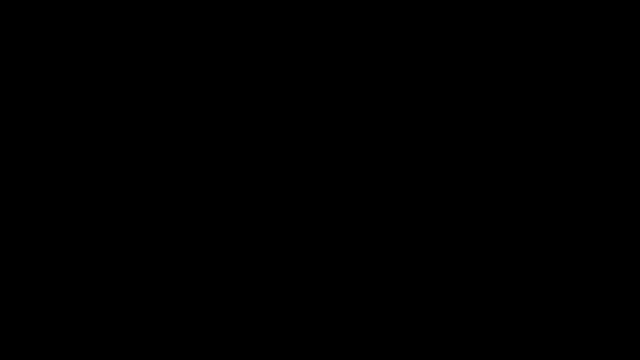 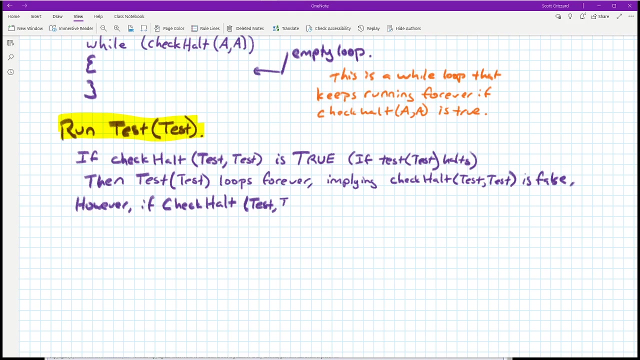 Yeah, Think about something else I could find and I'm going to make a scene. but when test, test up, Just as I'm getting to this point, I decided that I might be でВ to the punchline. I know, I know it's flickering. Just as I got to the punchline, it started. 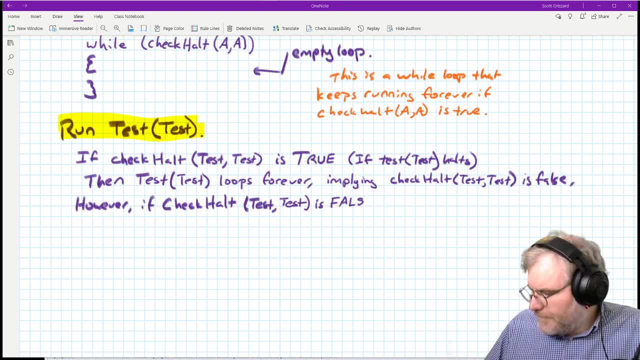 flickering again. However, if test test is false, then what happened? If test test loops forever, then test test halted. 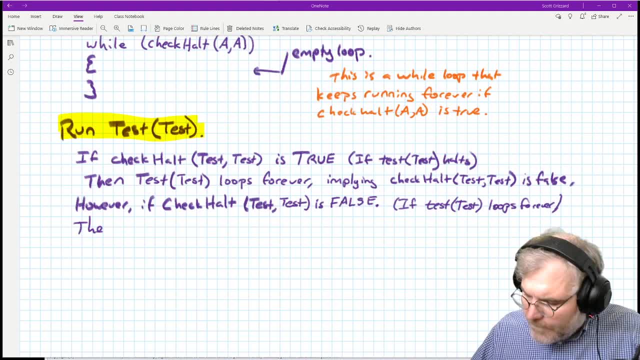 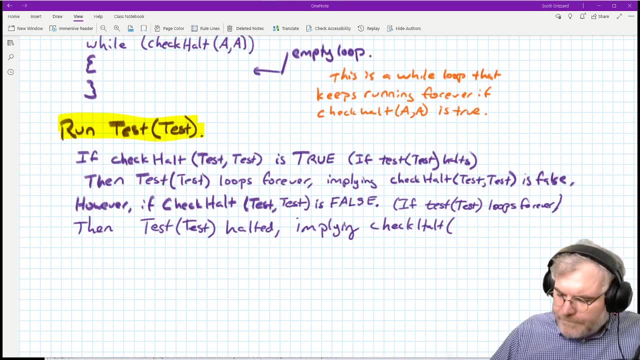 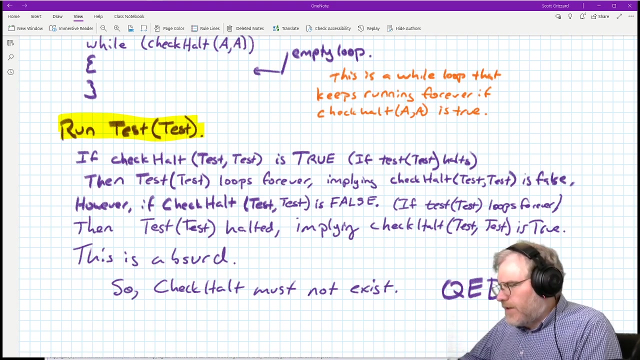 Okay, so how do we feel about that? one to five, Any questions. There should be a thousand questions. If your head doesn't hurt, I either did a really, really, really good job teaching. 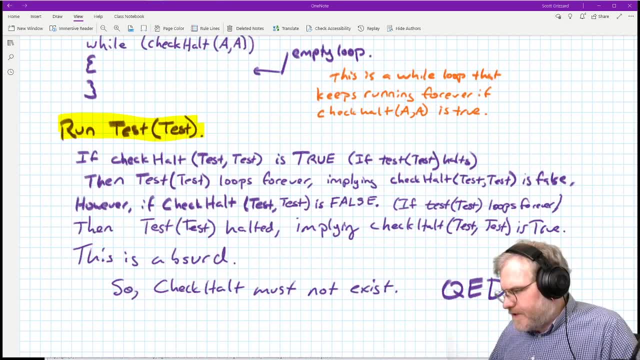 it- and I mean a better job teaching it than any other teacher I've ever seen it in the world- or you don't understand it, in which private case i didn't do a very good job. um, you know the? either the presentation was pro or you guys are praying, which is you know. 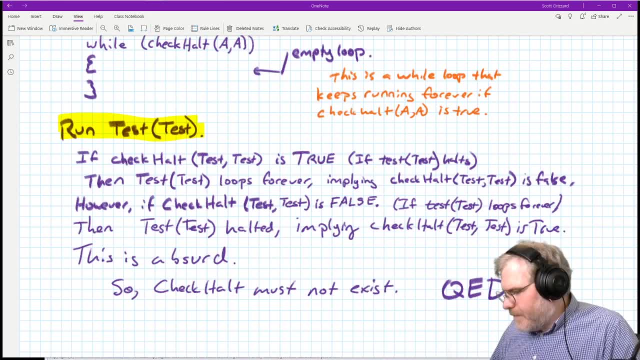 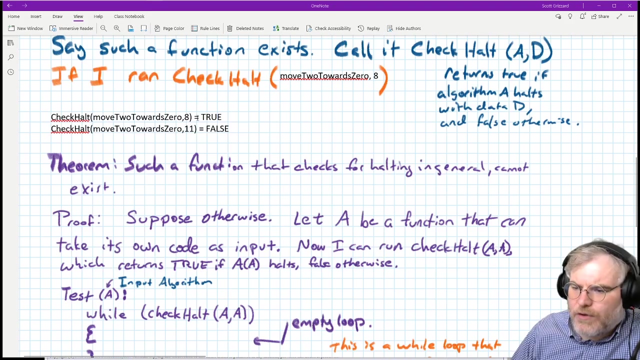 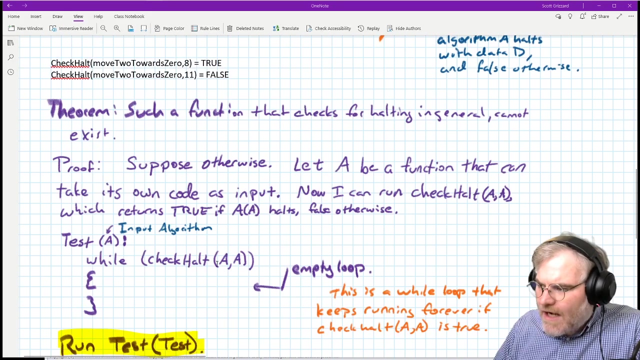 also possible. um, you guys are much smarter than me because this thing makes my head hurt a lot. so if you're going back to test, even okay, function named test, but your book used test, so i thought it was important to use test. test is the special function that halts if check. halt a a is true- i'm sorry, it's false- and it doesn't halt if 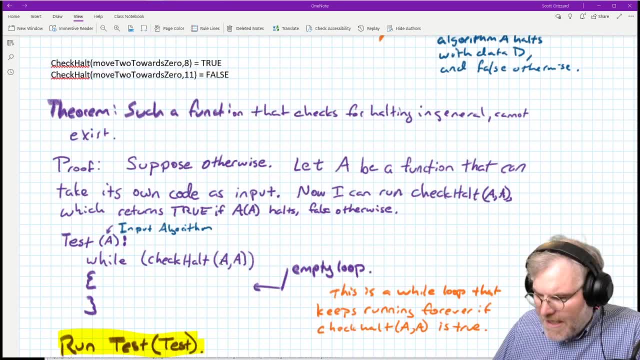 check: halt a. a was true, okay, and it doesn't. really. i hate the word the, the name test, but that's the one the book used, that i felt obligated to use it. you can use g as as the example if you want to. uh, the standard is to call it g, but the book called it this, so i was using this. 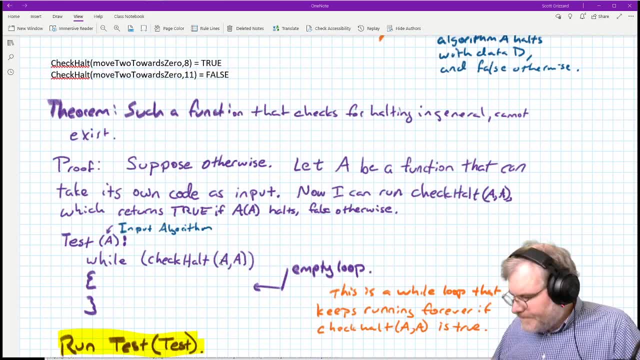 all right. okay, anyone want to take bets on test on plan b working for any length of time? no, there cannot be a program that that. okay. so when you hit alt control, delete on your computer what happens. okay. so if i come up here and i hit alt control, delete what's going to happen? well, everyone's. 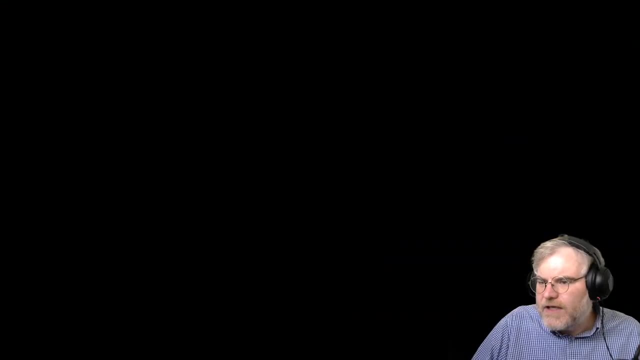 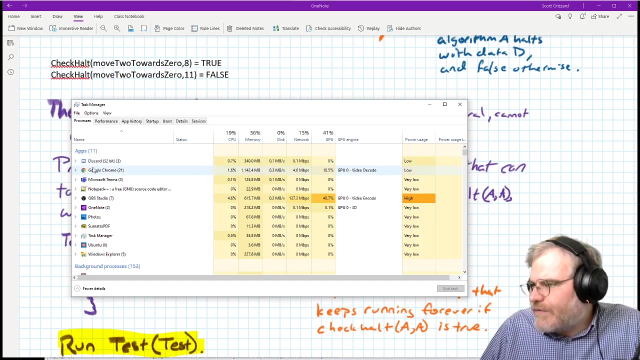 going to see me. you know, my computer go task manager and black screen, okay, and then the task manager comes up and the task manager tells me that this is running. i've got an instance of team running. i've got three messages on my teams. i've got obs studio running. i've got 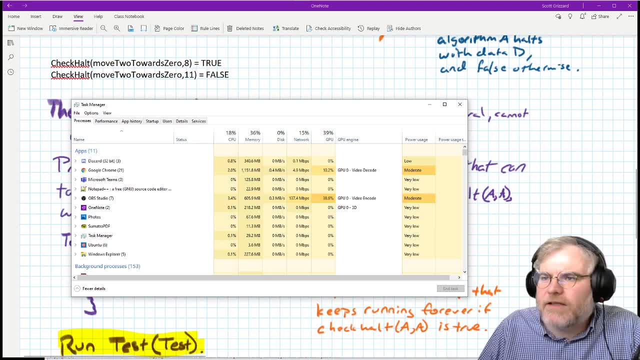 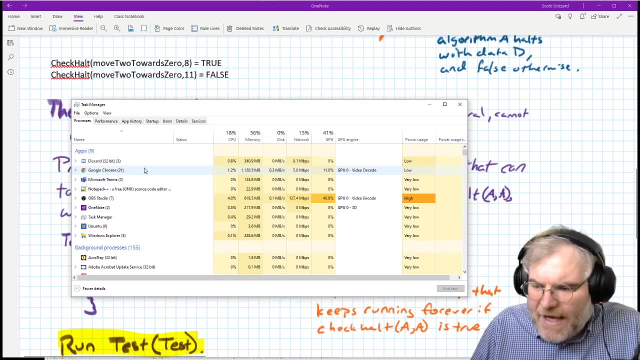 onenote running. i've got photos running. why is photos running? uh, i don't know why photos is running. um, i've got the pdf thing running, we'll get rid of it. and then i've got, you know, accutray, all the adobe stuff running in the background. okay, 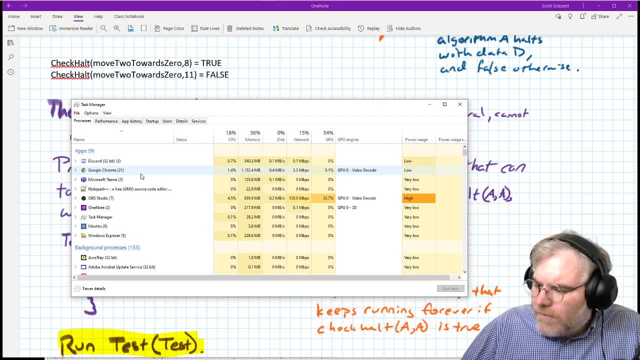 now all these programs are running in the background, and i've got all the programs running in the background, and i've got the pdf thing running in the background and i've got all the programs running in the background. okay, so is everyone on board with that? now, what this theorem tells me is that when this thing goes, you know, and if i started up skyrim- 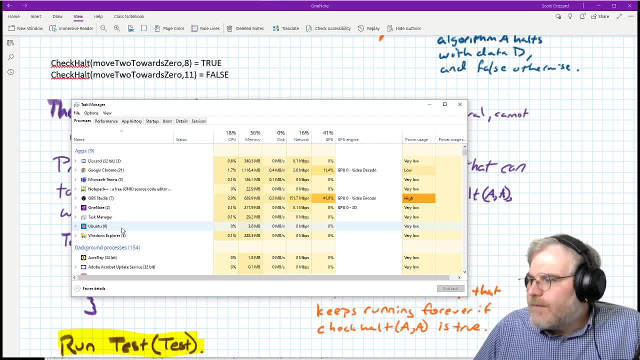 it would say: not responding, okay, because skyrim is sitting there in a loop loading itself, okay, but then eventually this not responding would go away. okay, but the computer can't tell if, the if, if a program is stuck in an infinite loop. that's the point. i can't actually check it if, the if the computer is stuck in an infinite loop. 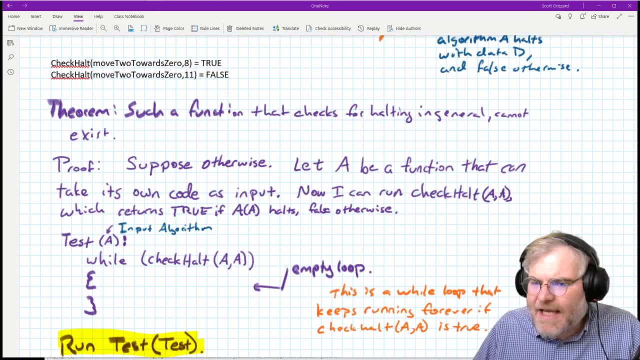 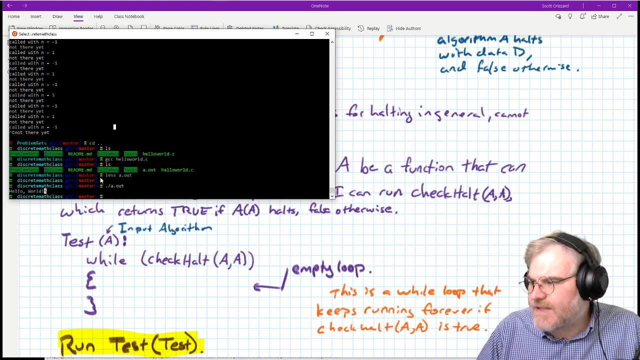 okay because it may finish what it's processing. the computer cannot tell the difference between stuck in an infinite loop and i've just got a lot of calculations to do. in other words, the computer cannot tell the difference in general. it can in specific instances, but the computer cannot tell the difference. 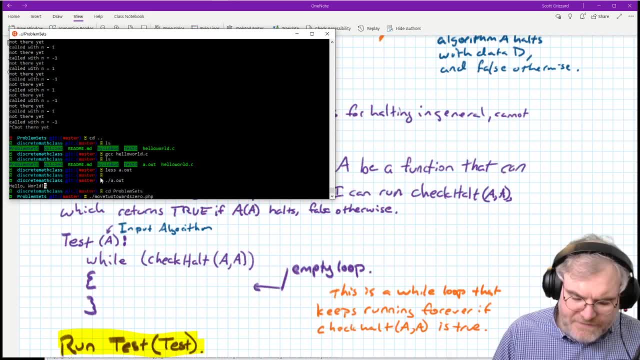 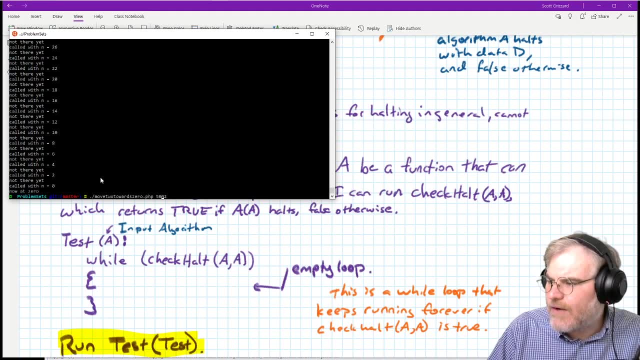 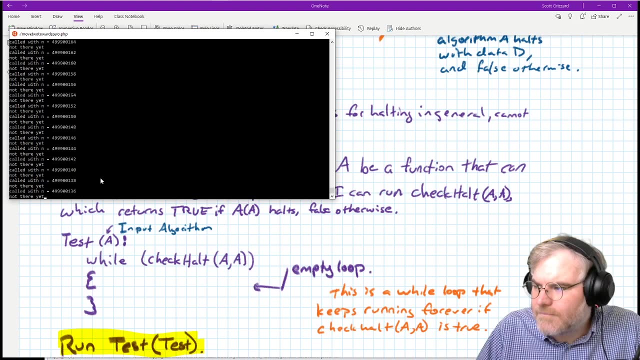 between this and this. okay, right, the computer cannot tell the difference between me asking it a really really, really, really really David number. okay, the computer cannot tell the difference between uh and this. okay, now, uh, uh is okay important about that. it cannot tell the difference whether or not. now, sometimes you can't, you can, you can. 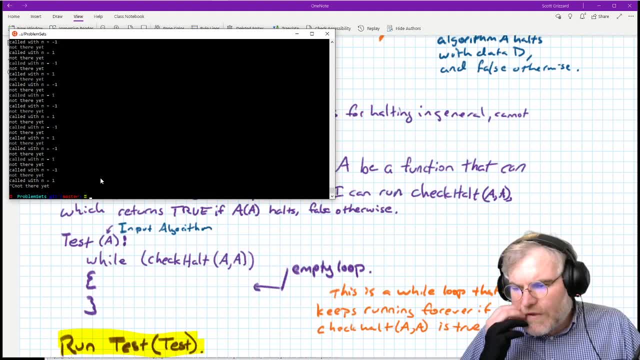 write things that that check for loopings in the, you can approximate it somehow, sometimes right. so like chess, okay, does anyone know that? there's a rule in chess that says if the same three rules get repeated, if the same set of of of moves get repeated, the same board configurations? 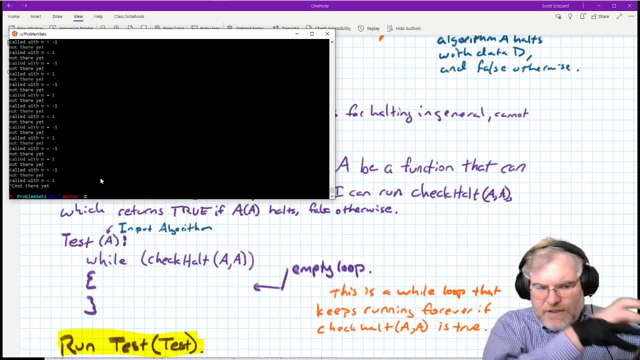 happen three times the same sequence of board configurations happen three times. that the game's a tie, okay, and that's the thing that the computer can check. the computer can't actually check to see if there's a way to break out of this loop or if the loop will eventually. 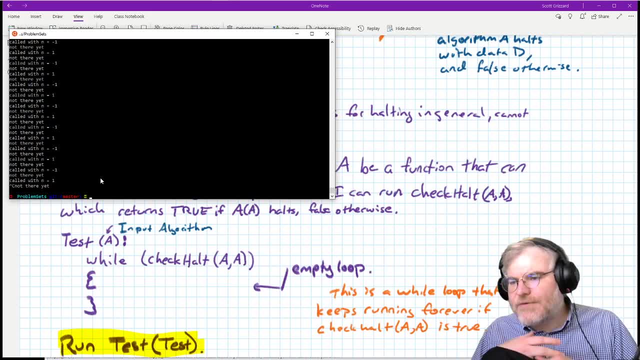 terminate. but the computer? the computer can do things like detect whether or not you've repeated x number of times, right? so i can't compute whether or not i've, i've, i've, i've run the exact same memory. i've run the exact same memory. i've run the exact same memory. i've run the exact same. 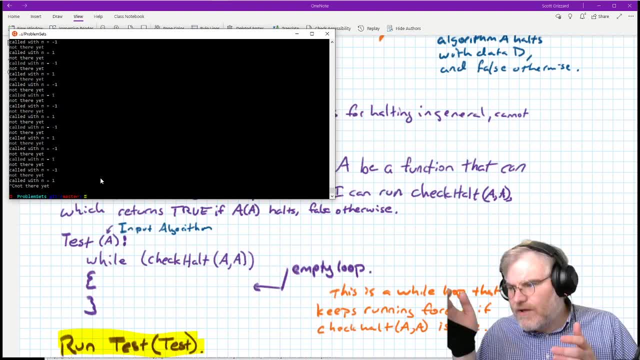 configuration ten times or whatever, but I can't tell that the algorithm is eventually going to break out, and that's the point. how do we feel about that? one to five, and that's the big piece here. so, one to five, we're probably going to end the class by crashing my computer. 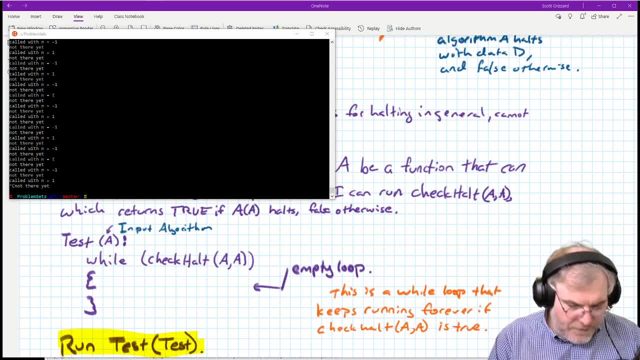 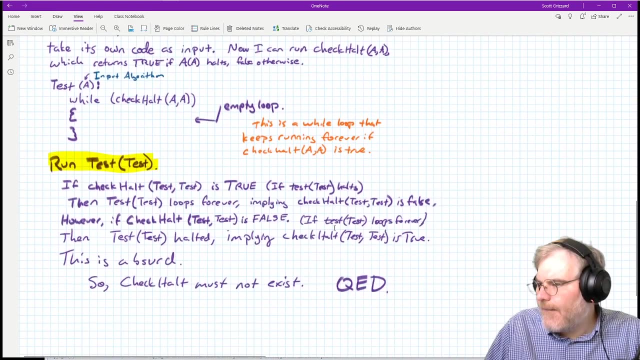 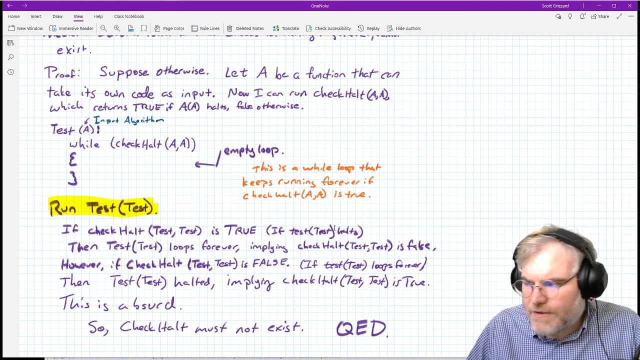 yes, but because it overheats or runs out of battery. oops, I need to fight bull. so one to five. how do we feel about this? it's weird and, as I said, if your head doesn't hurt you not really, you don't really understand it yet, or I'm just really really good, which is possible. 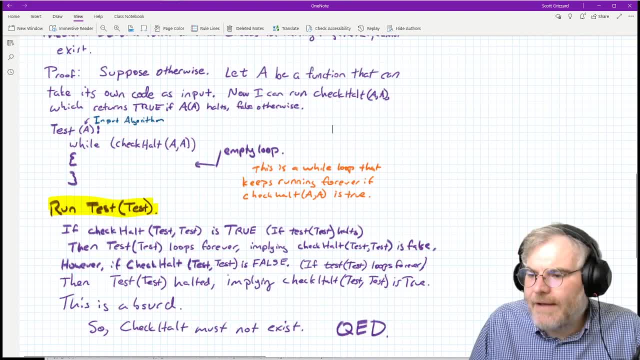 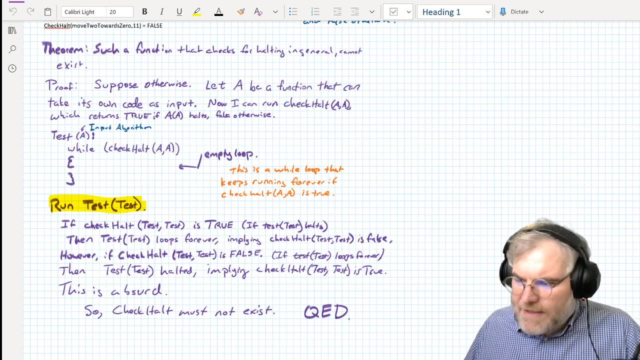 okay, so let's move on here a little bit. okay, now let's see if this thing works. all right, it's up. okay, so let's see if I get another 10 minutes. we got another 5- 10 reps. are we gonna have 15 minutes left in class? okay, so let's see if I can get. 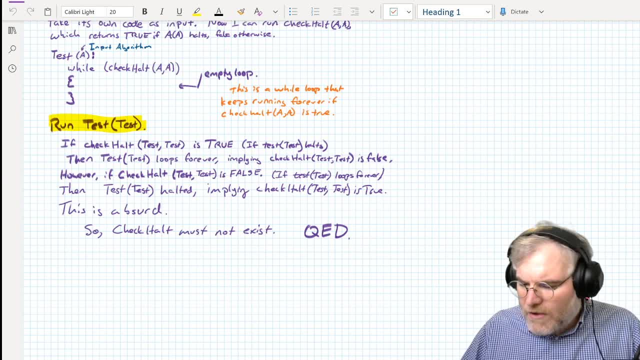 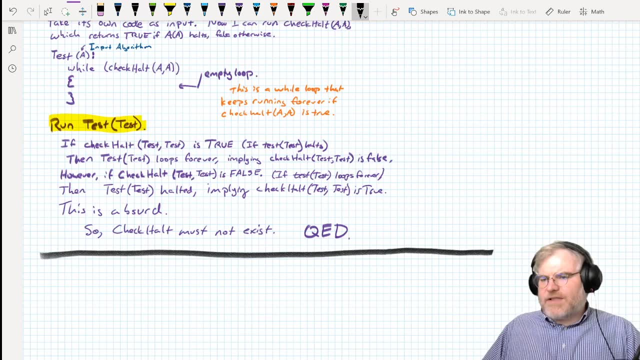 this computer to work Godel's incompleteness there. we're not going to prove it, but it's a direct it's. the proof is very similar, except I have to get around the fact that I'm using there Godel's incompleteness thing. math is a. 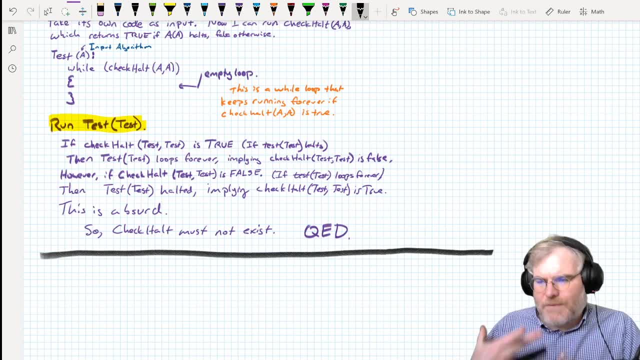 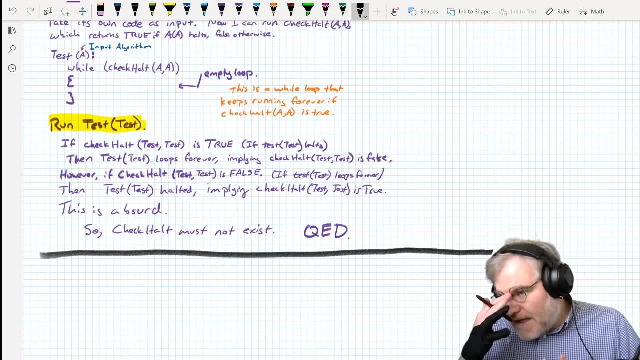 little bit more powerful. right, I can't enumerate over computer. a computer can't enumerate over something that's bigger than a countable set but- and in mathematics we have things called trimes, finite induction and stuff like this. so I actually can, under circumstances, certain circumstances, do things that talk. 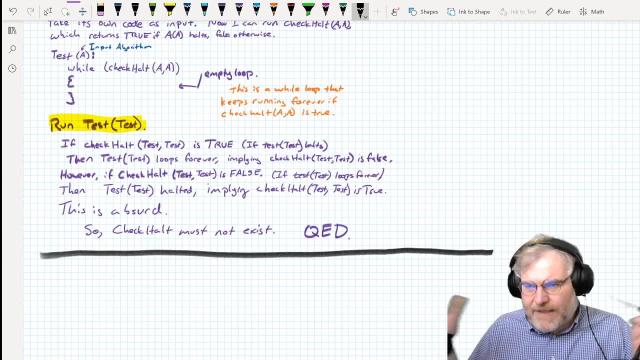 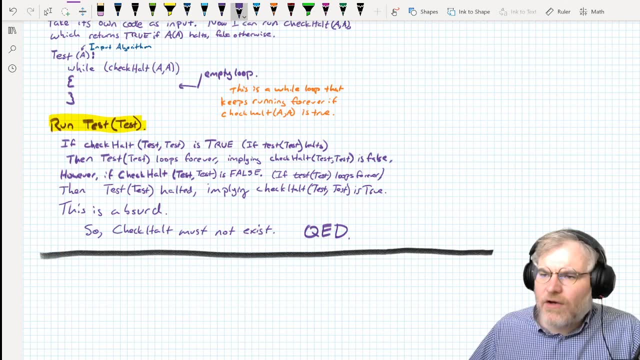 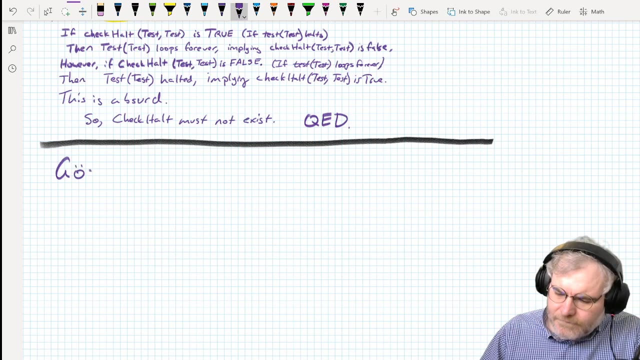 about things that are bigger than infinity, are bigger than countable infinity, bigger than the natural number. okay, but there's something called Godel's incompleteness there, and it's the same basic idea. maybe I can put in a number, I can put in a common denominator and I can put in a 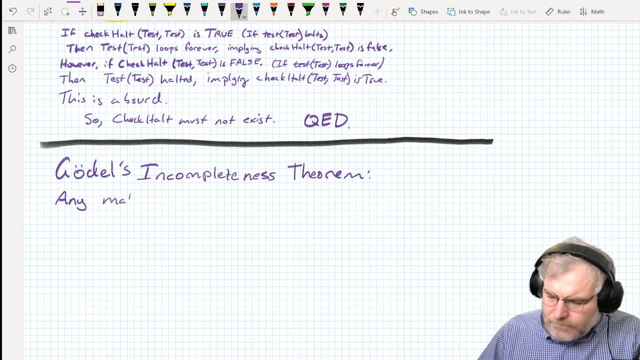 common denominator and then I can put in a common denominator and that's what I'm going to be able to prove. yes, so you got the key and you got the number, and you got the number pretty close to the answer to that, and then you can add a number. 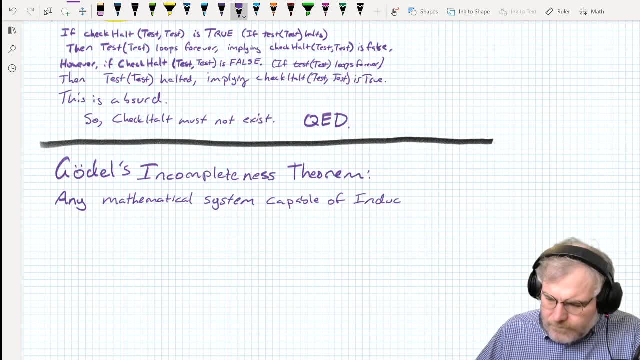 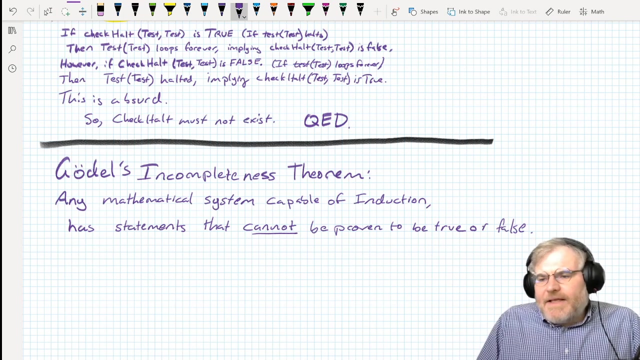 to that number. so now let's see if I can get this computer to work. all right, I told you I already did, and I know that's not a good idea, but you're going to have to give it a go. So Godel's Incompleteness Theorem says that any mathematical system 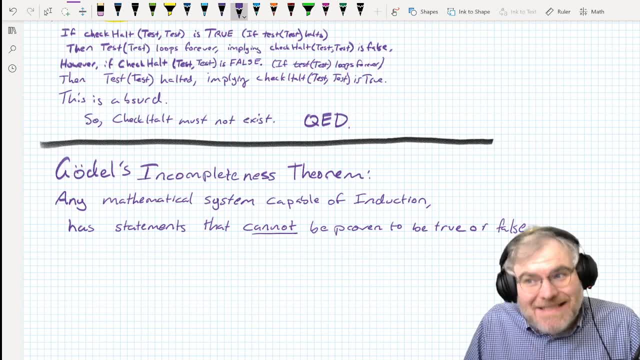 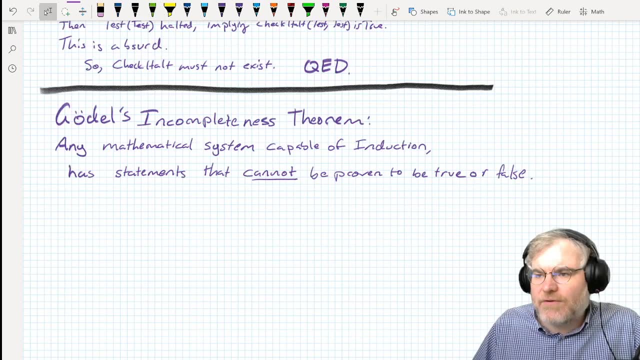 capable of induction. okay, in other words, any system capable of recursion- because, remember, they're the exact same thing- has statements that can be proven, neither true or false. okay, There are statements that cannot be proven. Oh, and one of these. 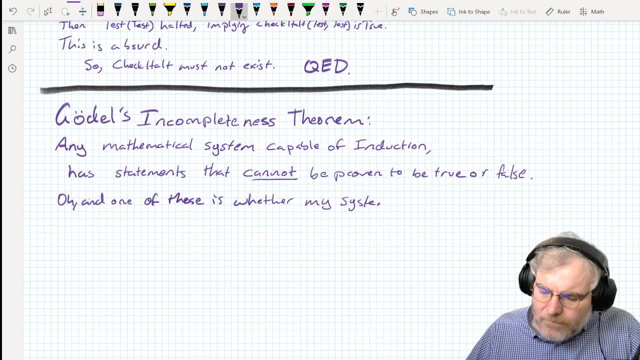 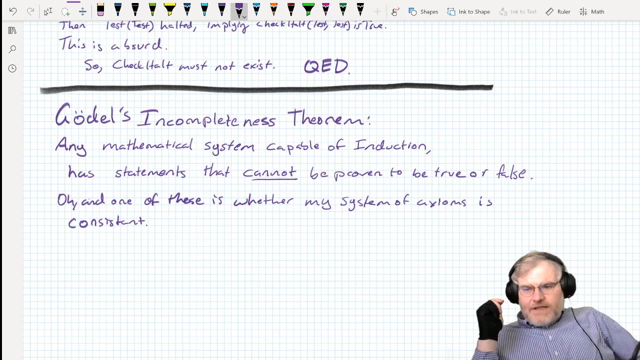 So, at the risk of sending you back to high school geometry flashbacks, at the risk of invoking high school geometry flashbacks, does everyone remember this idea that I have a sequence of axioms for geometry? I have things like two parallel lines, can never touch between any two points. 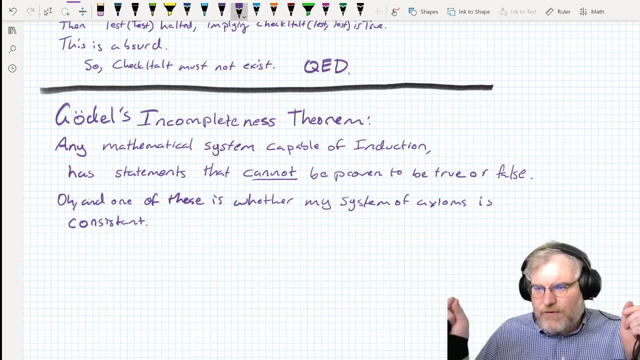 there exists one and only one line that passes between both points, right? Everyone remember these systems of high school geometry. Well, if I have a system of mathematics, right? if I have axioms, right? Yes, that says axioms. So if I have such a system of axioms, okay, I cannot prove. 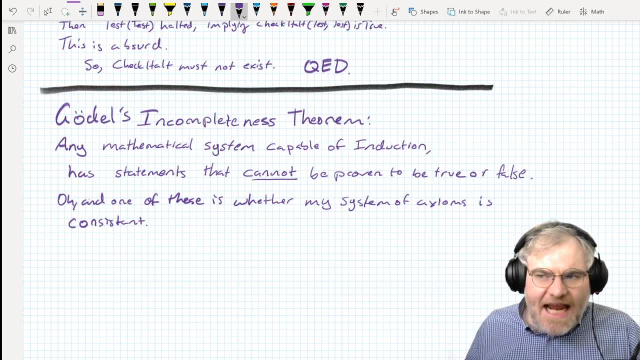 whether or not those axioms are consistent using the axioms themselves. as long as my system is powerful enough to do induction, as long as my system is capable of doing piano arithmetic, which is the technical term for it, my system I cannot prove using my. 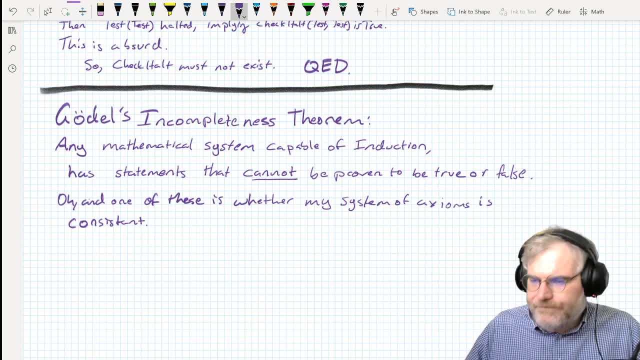 axioms, that my axioms are consistent. In other words, all the math is built on sand. We're pretty sure about it, but this is where mathematics has to go off and tell philosophy. okay, you have a job now, right? 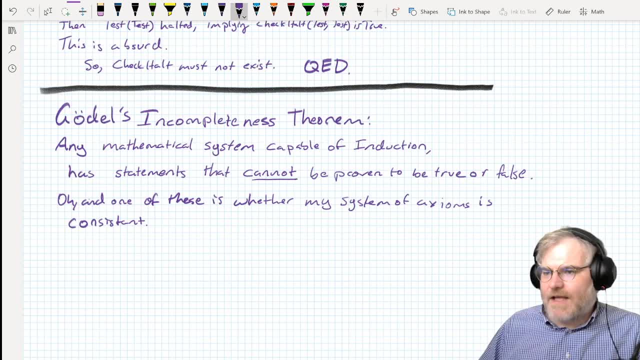 Talk about these things philosophically because we can't actually prove they are consistent, And it's important to note that the system has come crashing down on us twice, So the entire system came crashing down when people started doing non-Euclidean geometries. 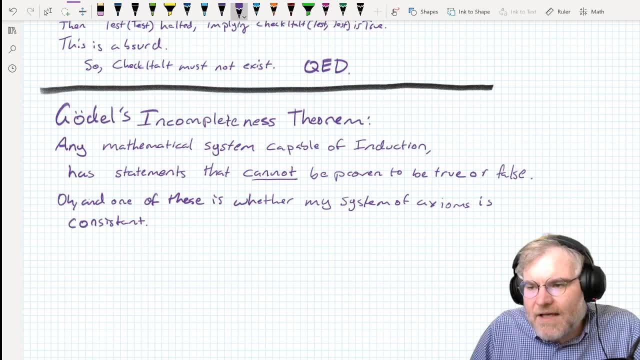 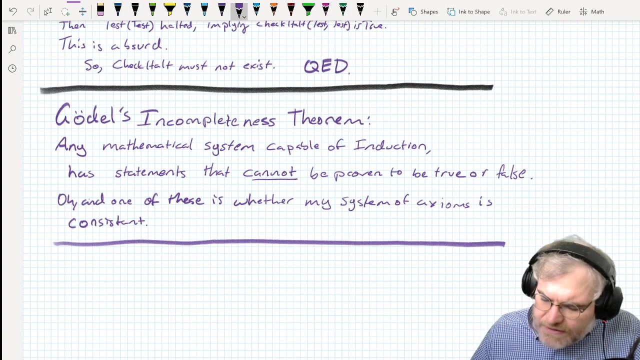 and then the entire system came crashing down when Russell stated Russell's paradox. Are there any other questions about this? Okay, Any questions, comments, issues, suggestions, thoughts, Okay, So the first thing is that there is homework. so there is homework on. 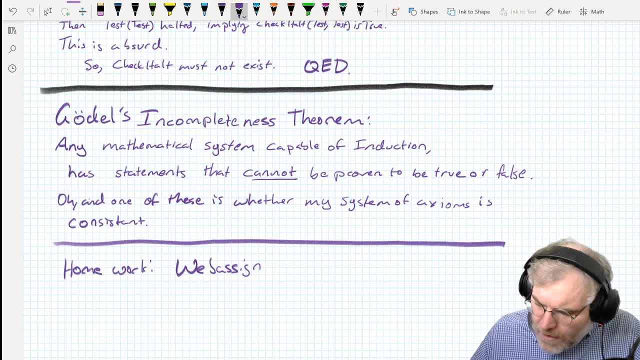 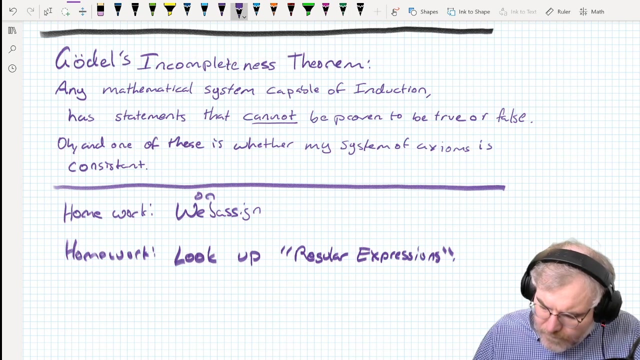 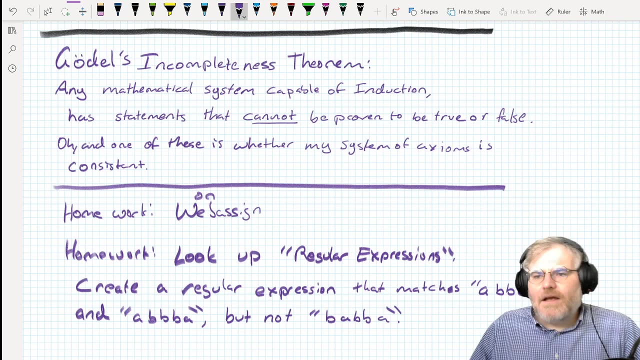 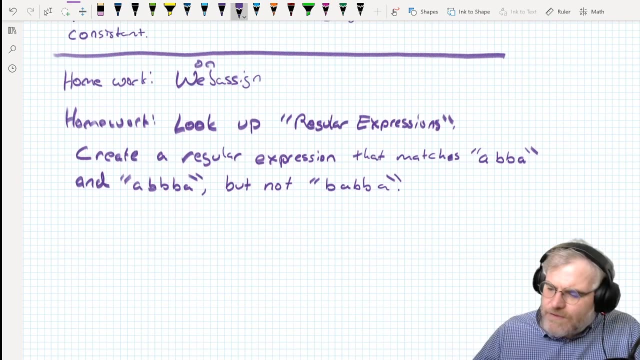 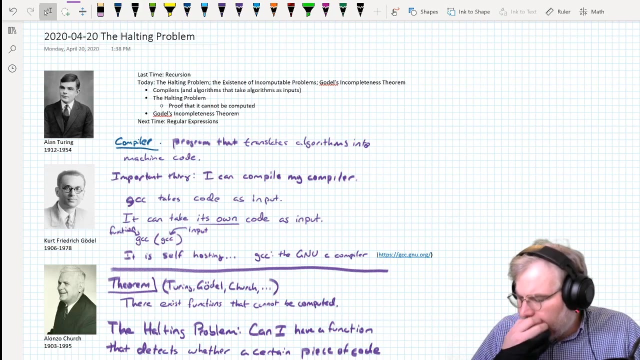 the network on the website, on webassign. that is due Tuesday, so tomorrow, and the other piece of homework is this: Google or look up: